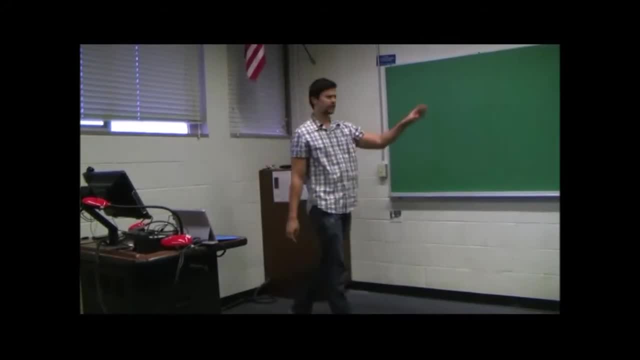 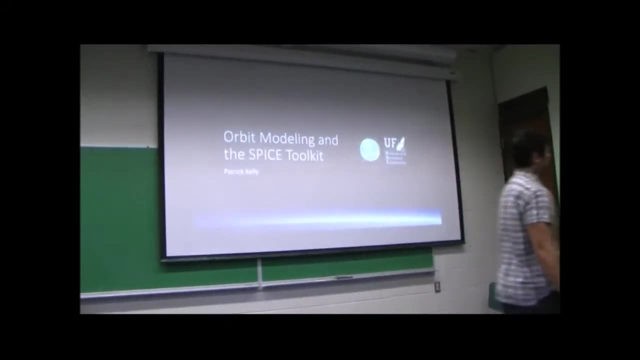 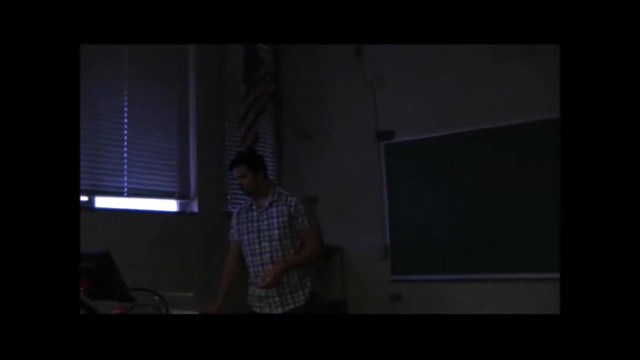 Okay, can everybody see this? okay, Do we want lights? more lights off. Yeah, Cool, Is that better? All right, Okay, so, like Dr Bev Block said, I'm going to be talking about the SPICE Toolkit. 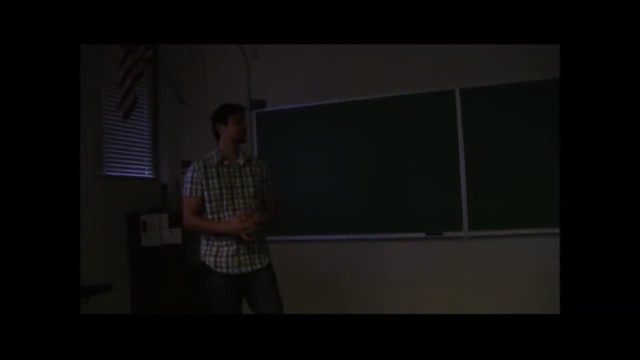 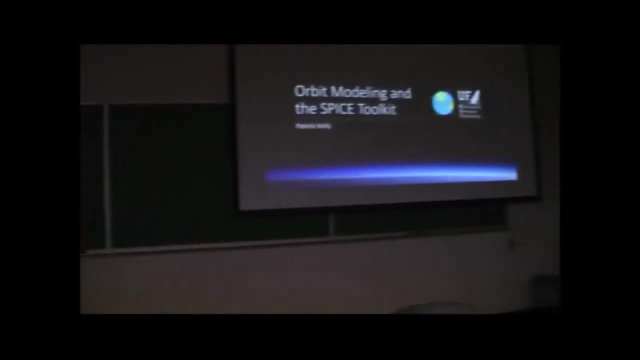 And it's basically it's developed by NASA. It gives you a lot of information regarding the planetary constants, the ephemerides, a lot of information on various spacecraft that they track, And I'll go into more detail in a second, But first we're going to talk about kind of the basics of orbit modeling. 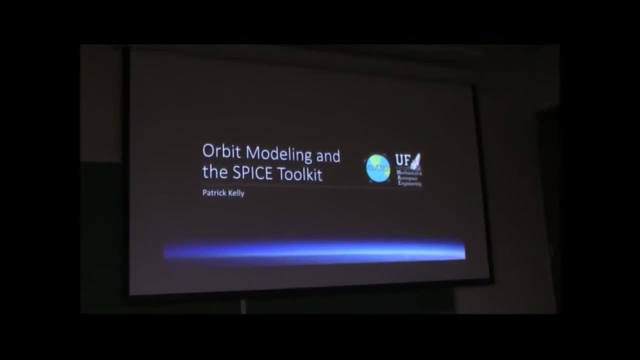 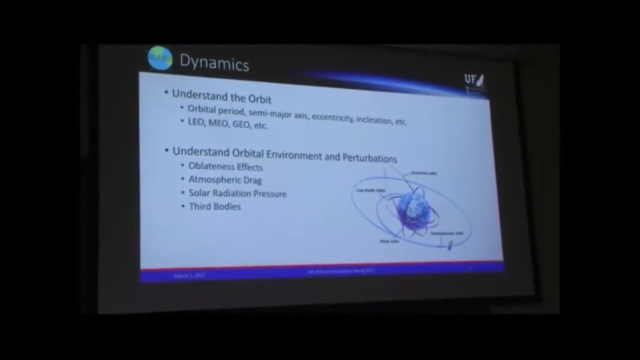 Because this is basically going to assist you in making your own kind of simulations on MATLAB- or mostly MATLAB we're going to be talking about today. So first of all, when we start talking about creating our own simulations, we want to have a good understanding of the dynamics that are involved with our simulations. 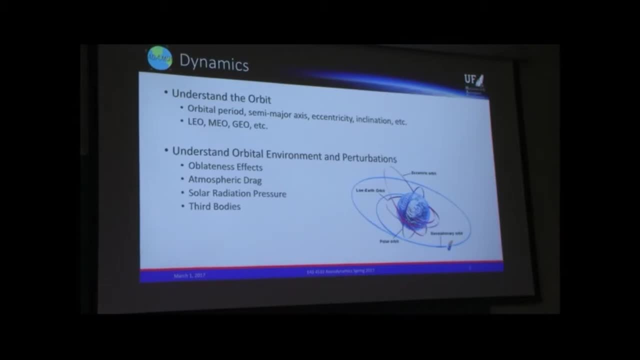 So if you have a mission in mind, you want to keep a couple of things in mind when you start programming And throughout the entire simulation you want to kind of know the behavior of your satellite. So it's good to understand, you know, the orbital period of your satellite, the basics, like the orbital elements. 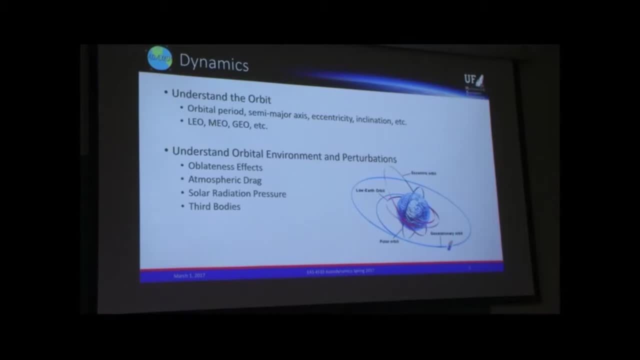 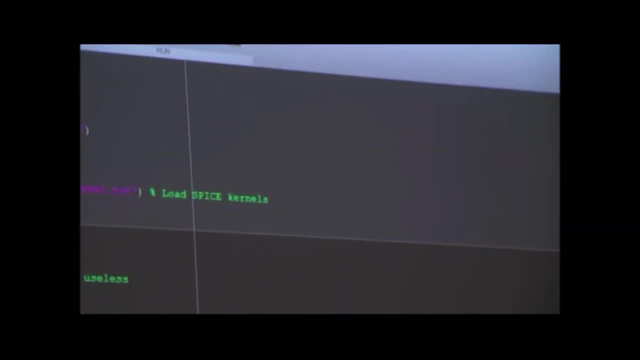 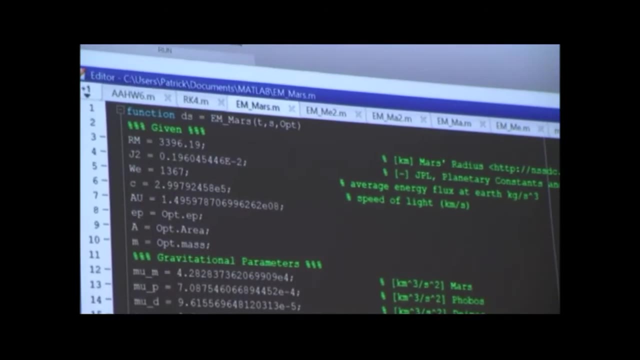 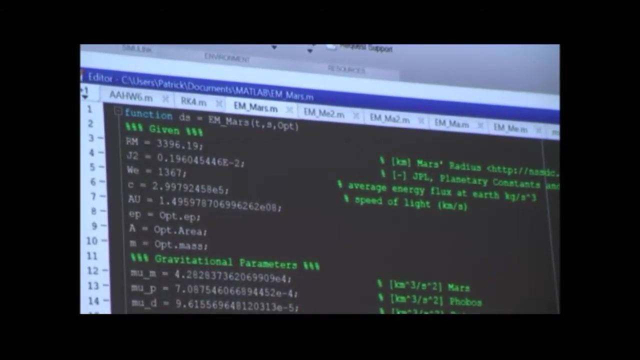 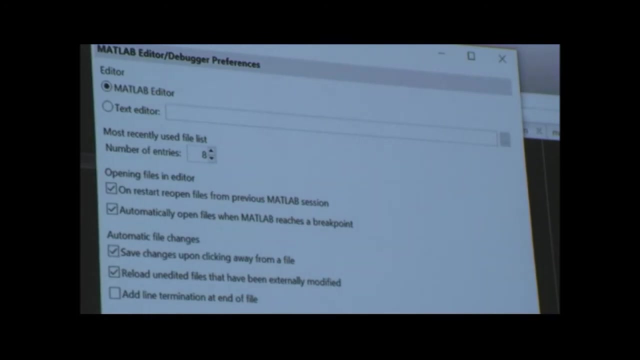 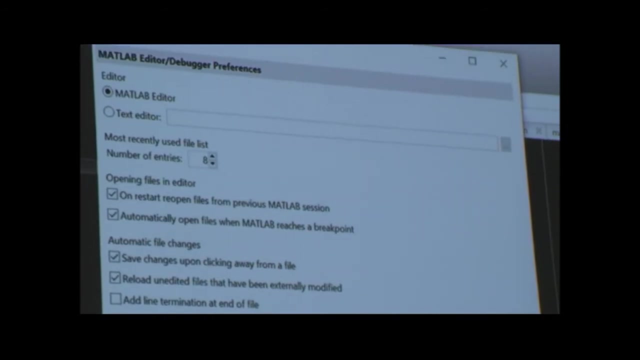 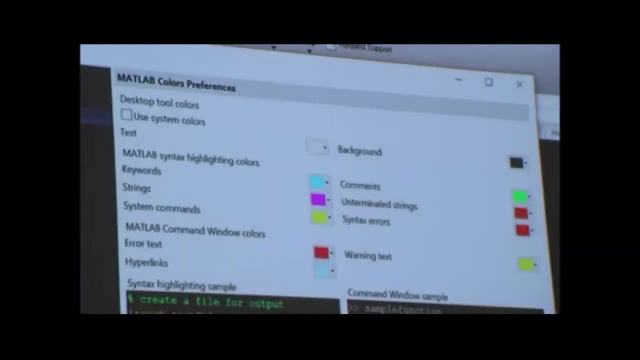 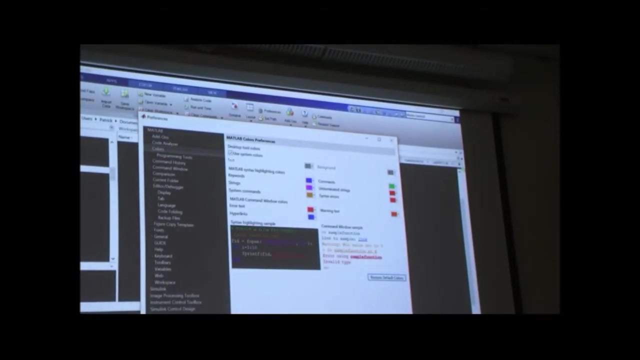 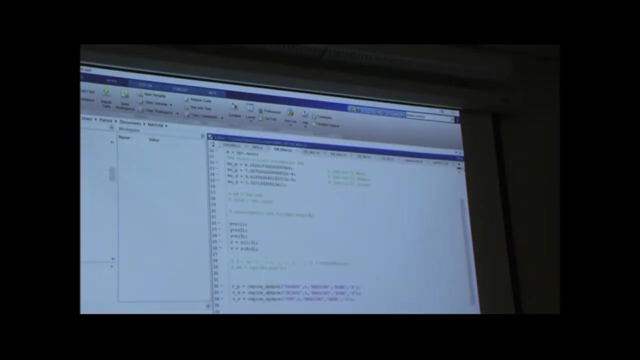 I'll change it back. it won't take long. well, it shouldn't take long. I don't know why it's freezing up Computer at stage fright. there we go, Must be. Alright, let's call it Mars, MiceMars. 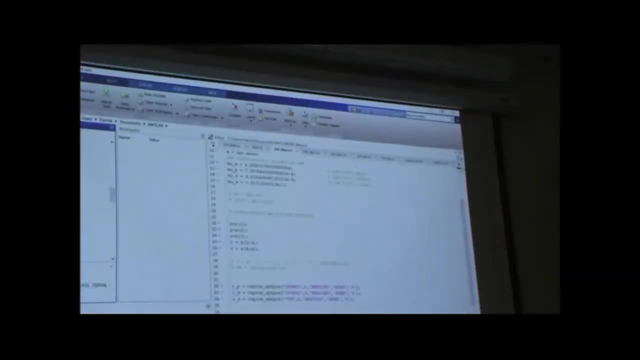 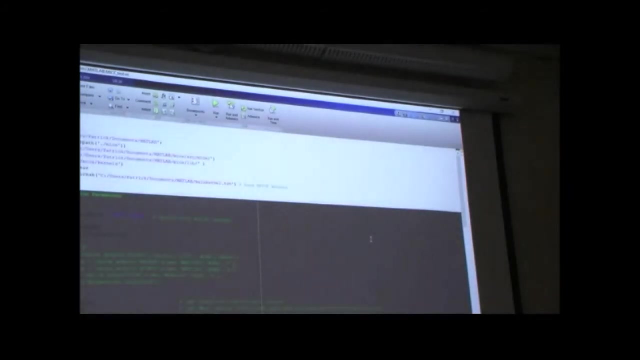 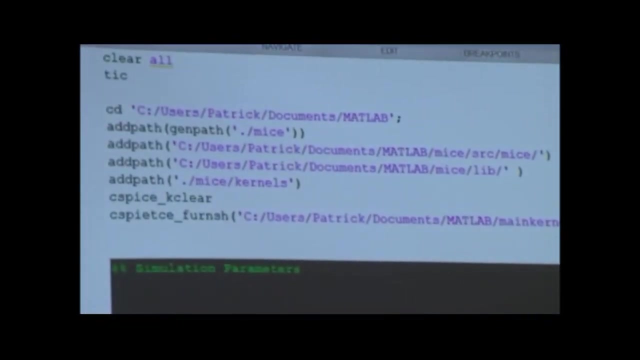 There we go, There we go. Oh well, alright, we're going to have to deal with it. Okay, so the first thing I did here, like I said in the presentation, I'm going to go ahead and load the. 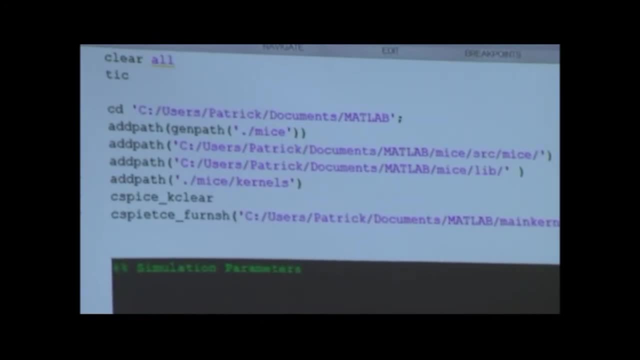 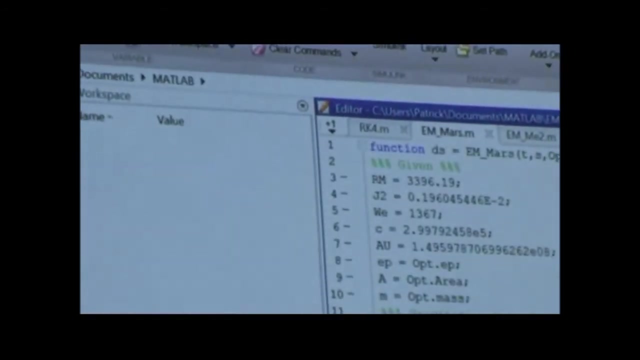 The spice toolkit. So I add this mice folder to the directory, I add this library folder to the directory and then I'm creating a path to where I'm storing all my kernels, And I'll show you what the kernels look like as well. 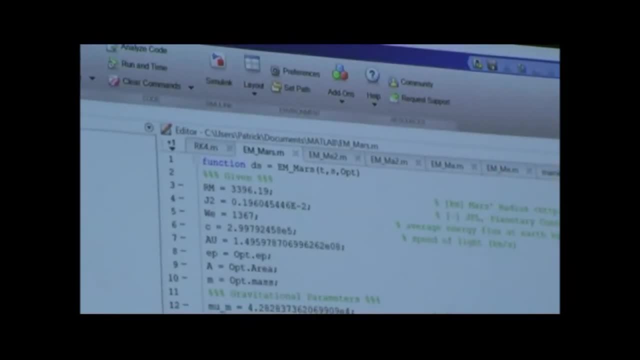 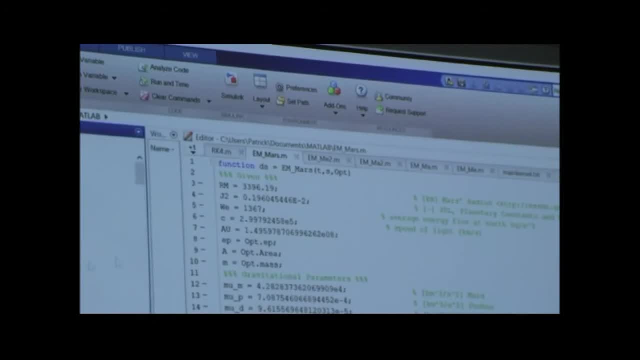 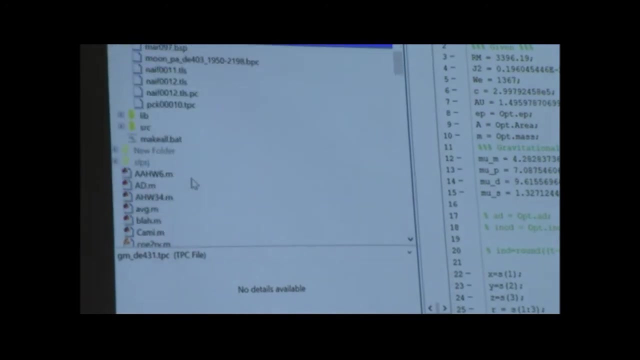 So they all have kind of goofy names like DE-430 BSP- This is a MARS colonel- MAR-97 BSP and you can't really read them. If you try to open them up, it's going to be: 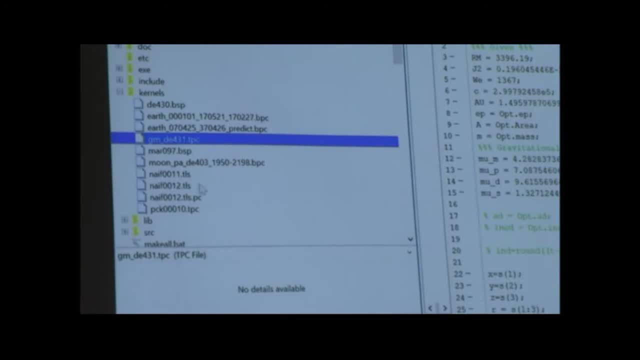 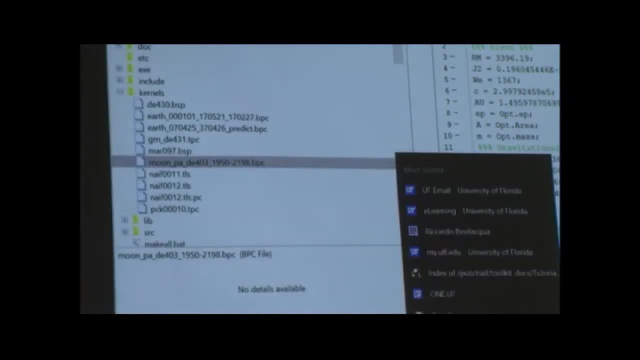 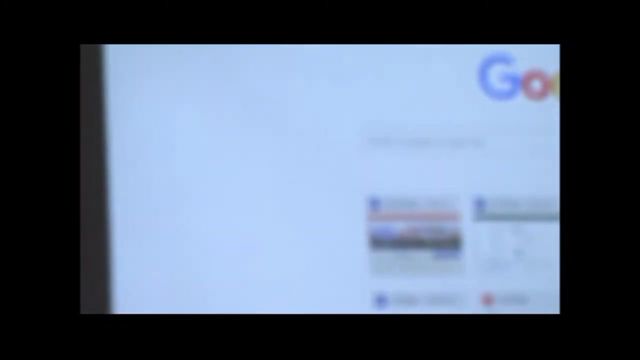 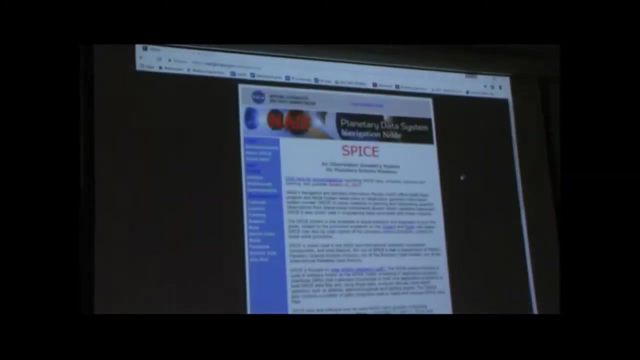 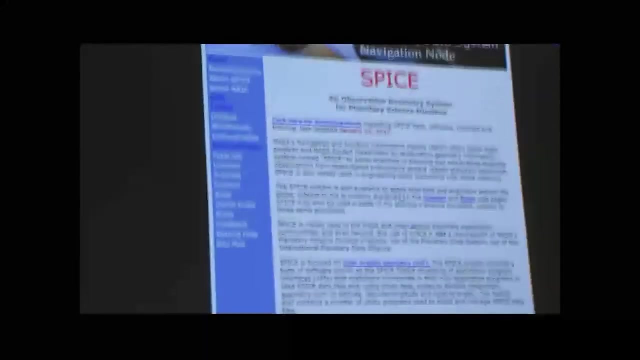 So those are the ones that contain position information as a function of time, for example. Yes, You pull this from knife whips. Yes, So this is the website. This is the site that you'll be looking at to get this toolkit installed. 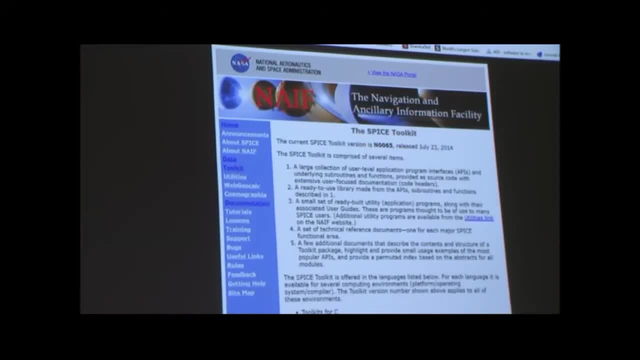 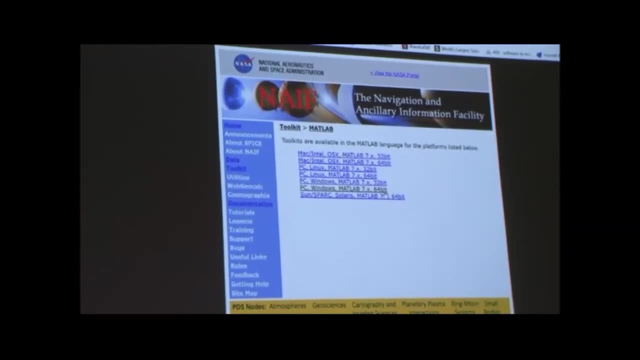 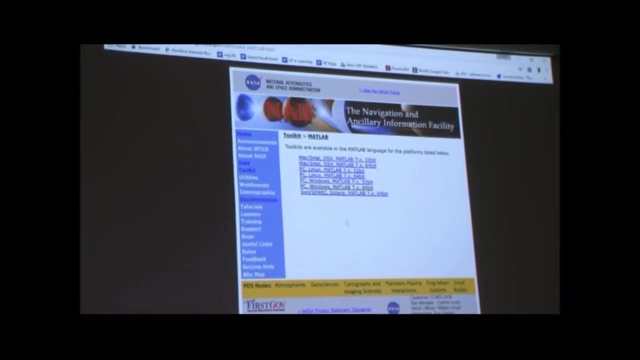 Just go to Toolkit, MATLAB down here, and then, if you've got a 32-bit, you'll click this 64-bit. maybe you're running on a Mac. you'll use one of these links. So when you run these you'll find the kernels on your computer that will be installed. 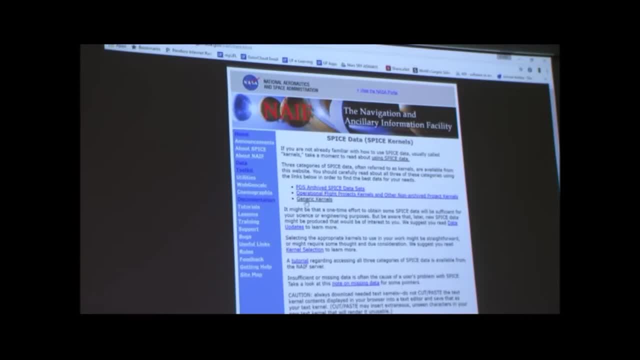 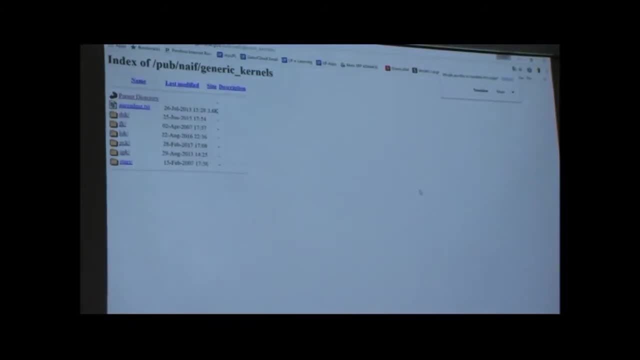 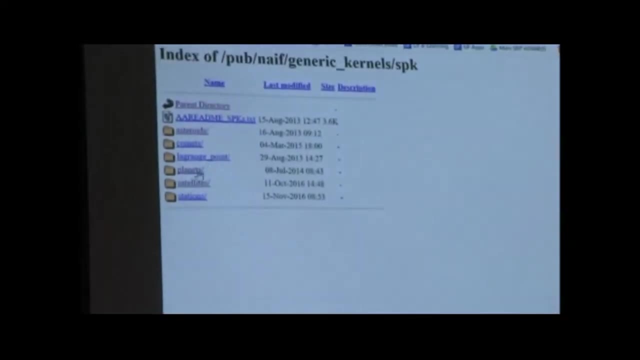 So, yes, And the kernels come from this data tab here. Okay, Okay, Okay. So I'm going to give you an idea of how fun this website looks. So you're going to be pulling from something like this, And if I want something with the planets, I'll click on planets and then ta-da. 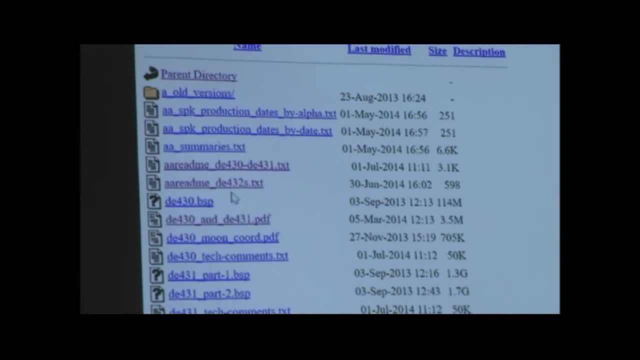 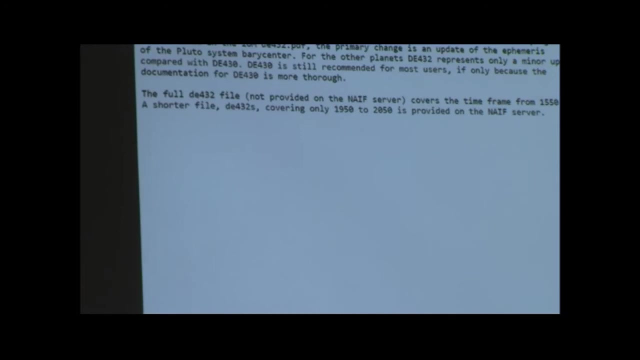 These are your kernels And then, if you want to know which kernel to click, you find one of these text files. Maybe I'm interested in 432.. Let me see. Let me see what that one's about. Read this: How long are they current for, as this is from 14,, you know. 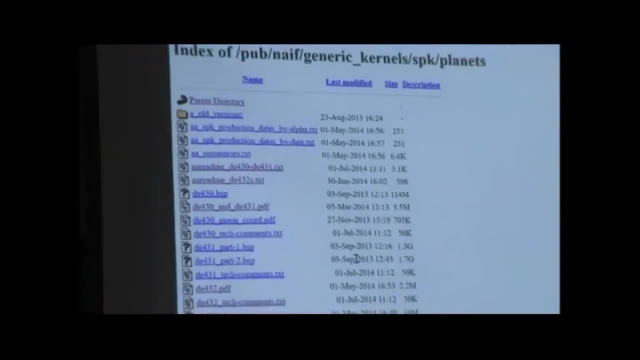 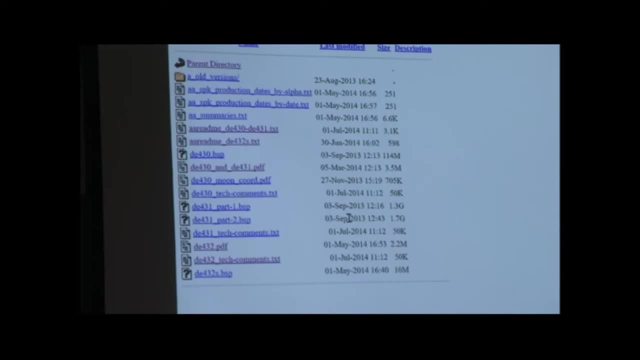 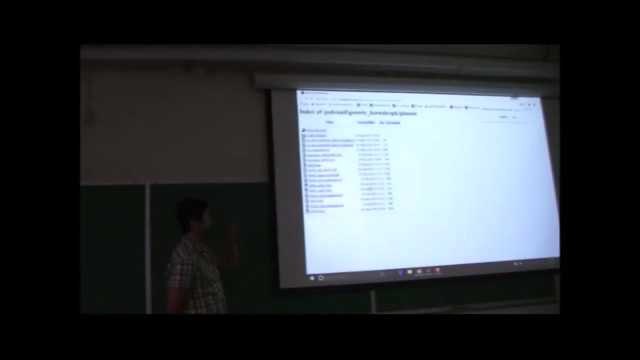 They recently did some updates, A lot of the support information. they have tutorials and PDFs and instructionals. They updated those this past January, so there's some updates regarding how to use this software. But these kernel files can be as old as. 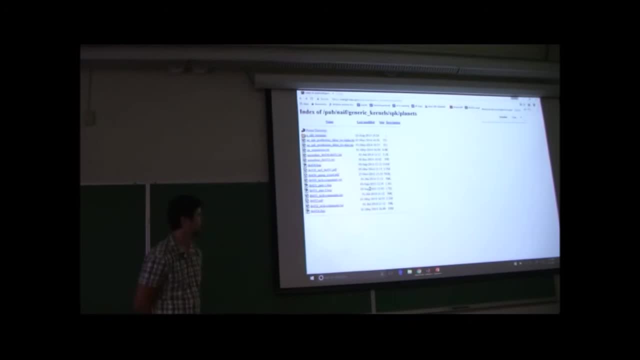 You know they update them as necessary. So, yeah, it looks like these are around 2014,- 2013.. But these are the most up-to-date. So these are the ones you're going to pull from, But it can get kind of tricky if you want to know which kernel to download. 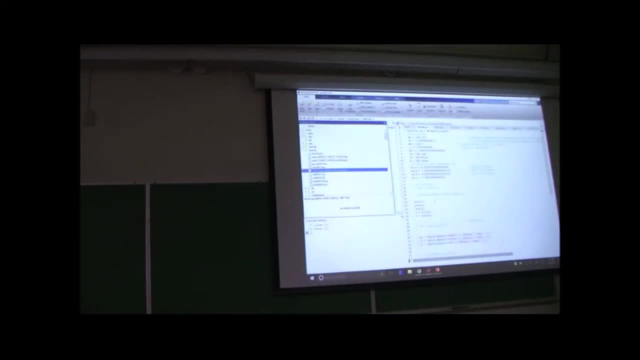 But we'll play with that on our own time. Okay, So back to the simulation. Okay, Okay. So you downloaded all those kernels. I'm going to show you the kernel, the meta-kernel. sorry, Let's go up here to MySQL. 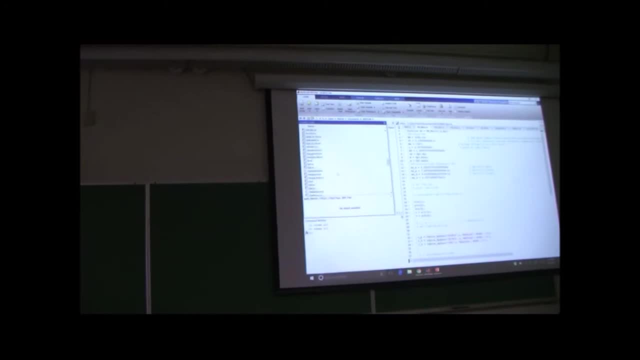 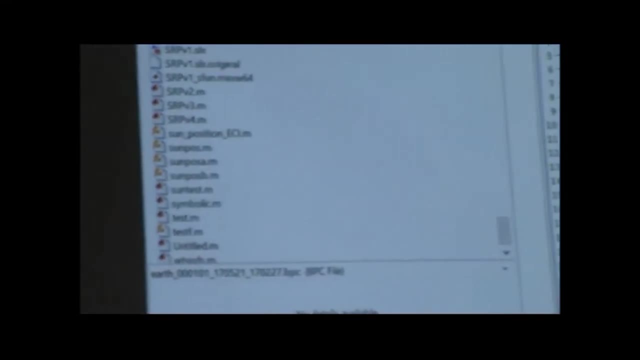 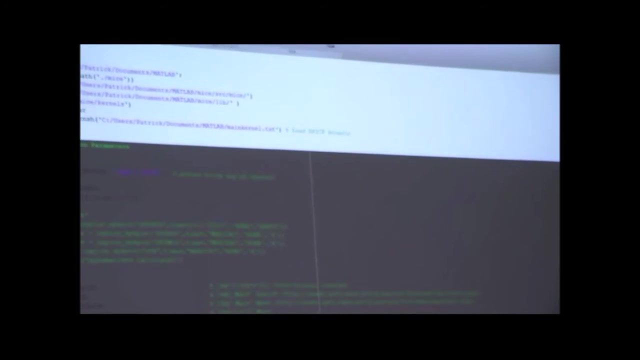 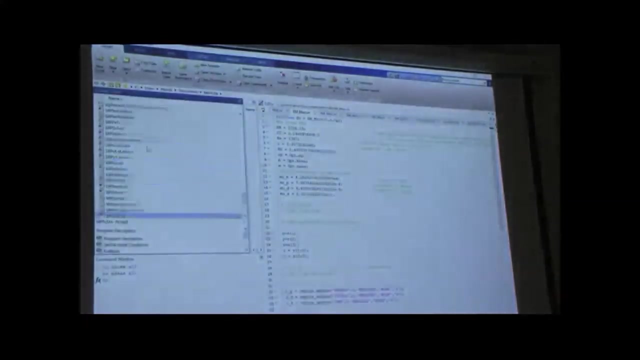 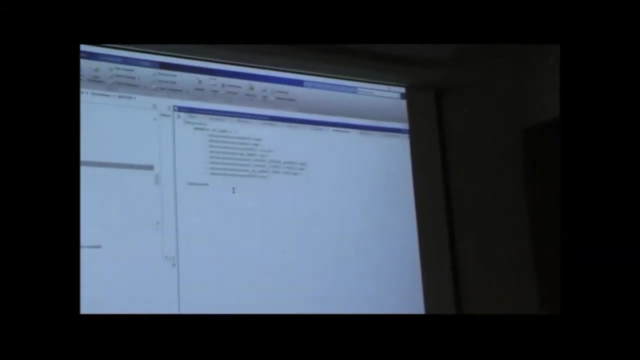 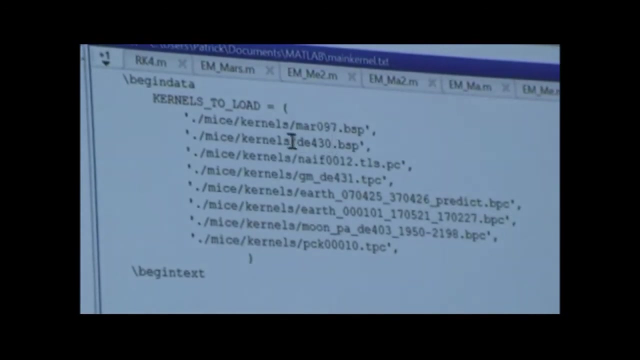 There's all this stuff. God give you an idea of what this kernel looks like that I'm loading Genpath, MICE, library, MICE kernel. So here's my meta kernel. I've got a number of kernels loaded up. I have a Mars kernel. This is a. this is 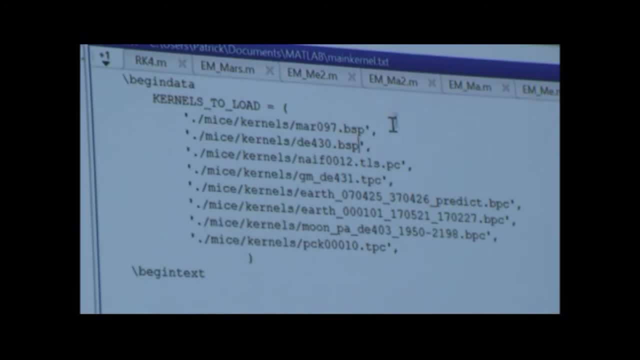 the main kernel. It has information for all the planets, some asteroids. This is the latest time kernel, So this will have updates on how to convert a string, a date string, to the accurate number of leap seconds past J2000, if I want And 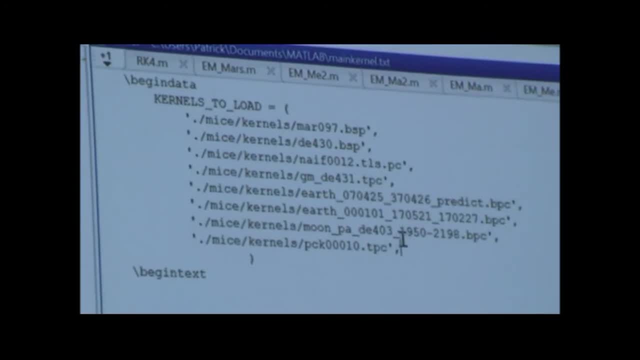 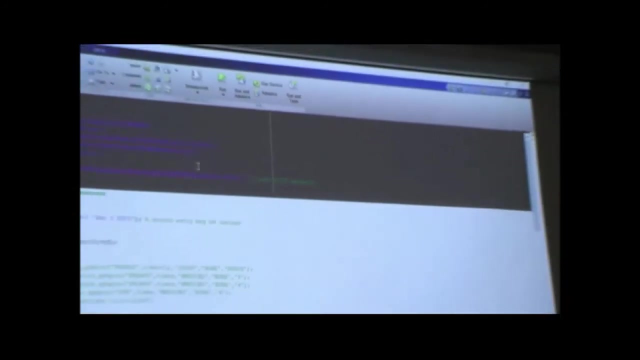 these are. these are specific to some research I'm doing, But this one has to do with the moon position, Earth's position And this. this kernel here talks about the gravitational parameters and frame information for various different reference frames. So I'm going to start the simulation at January 1st 2015.. So I can go ahead and 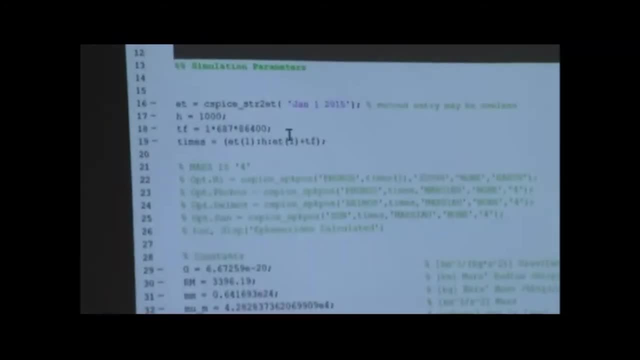 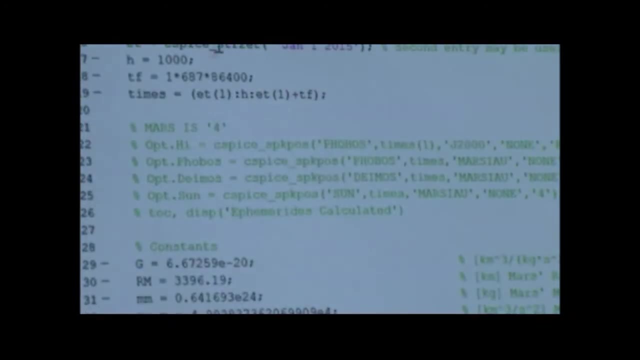 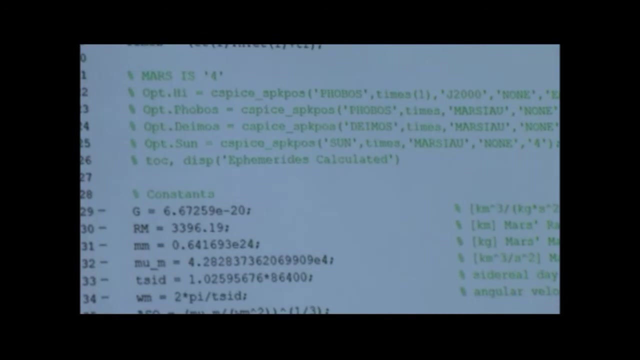 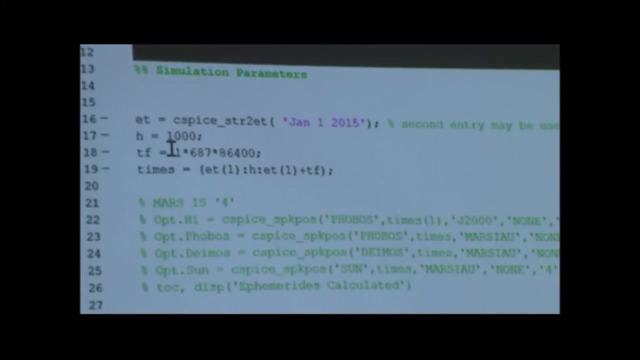 just type it in like this And I input it to the C-spot And here's the result. And so I'm going to add up the string here And I'm going to add up the variable variable and the primary code for that. So I'm just going to add i2 string to et right here. This is: this is a variable. I'm calling time. final is basically going to tell me how long I'm running my simulation. A martian year is 687 days, So this one is just going to add 687 days to whatever my initial time is. So if my initial time is January 1st 2015,, 687 days later, if my initial time is January 1st 2015,, 687 days later, 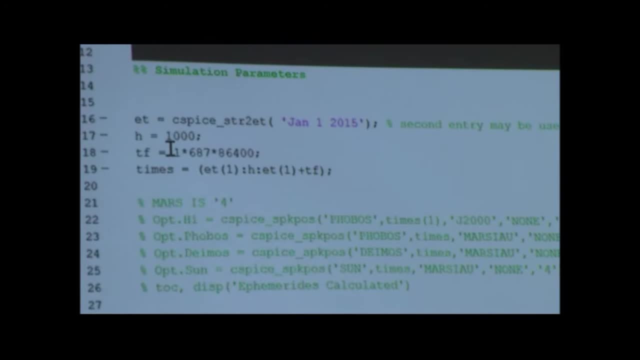 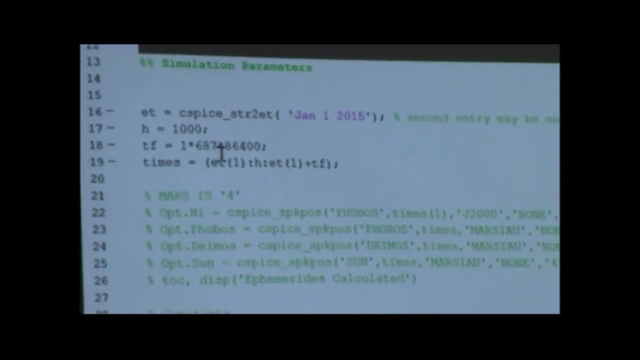 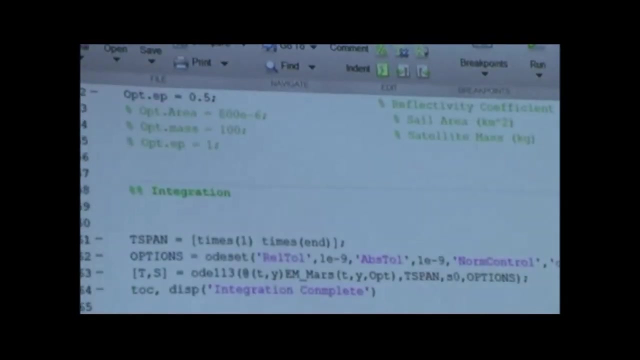 That's where my information will stop for the time information I pull from Cspice, It will pull basically that window of time instead of pulling all the time information it has. First of all, I'm going to pretend I put the ISS at Mars, Why not? 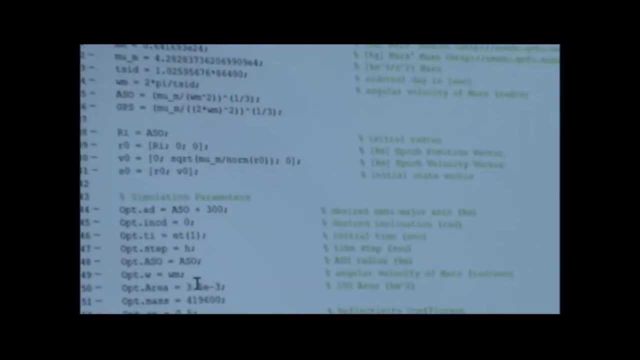 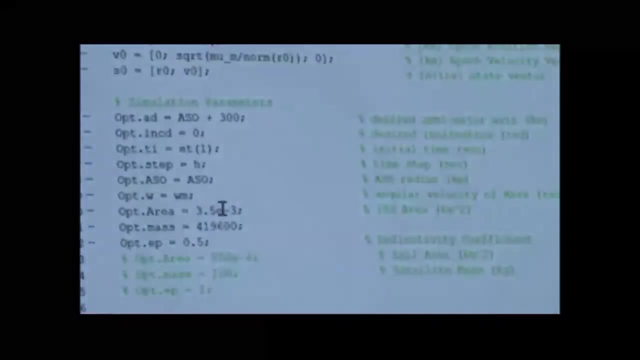 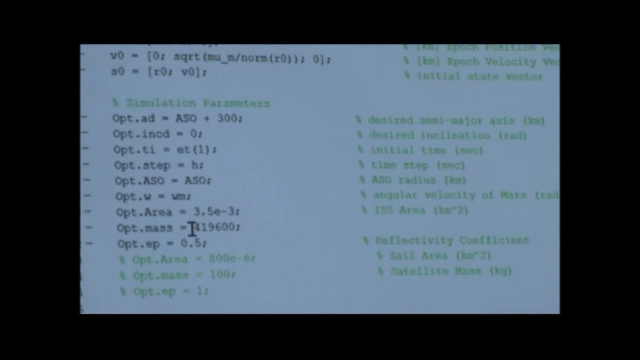 I'm assuming the ISS has a surface area of about 0.0035 square kilometers. on average It's got a mass of 419,000 kilograms. I'm going to simulate an orbit around Mars. that's about 17,000 kilometers. 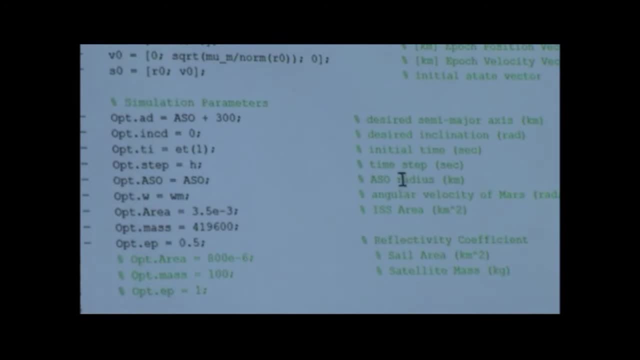 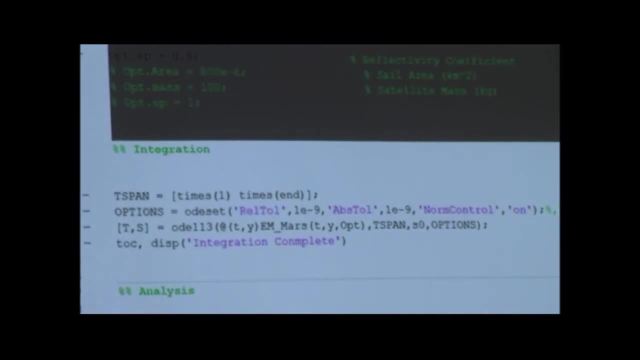 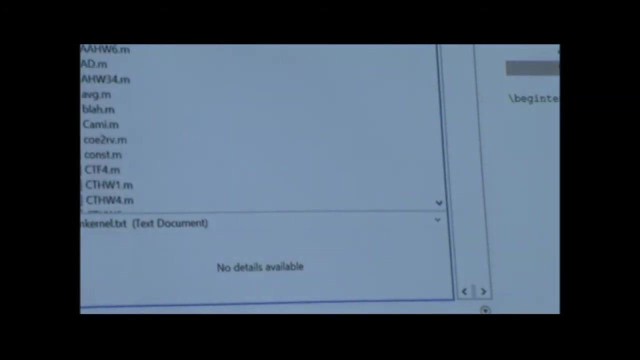 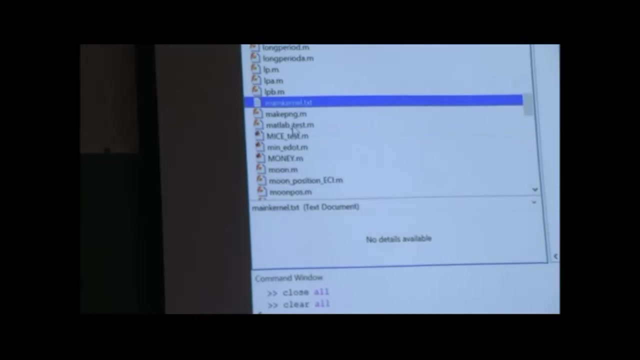 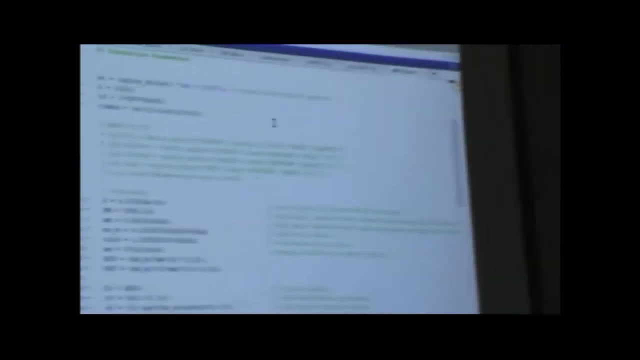 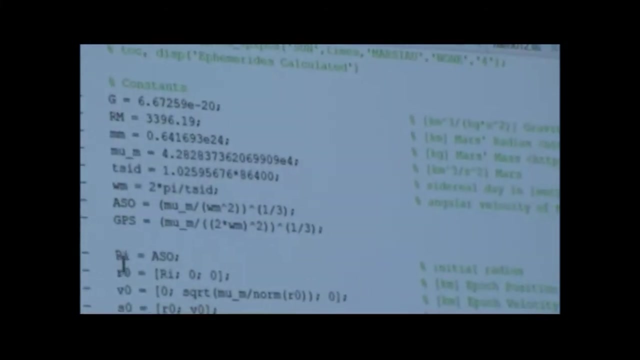 17,000 kilometers from the center of the planet. I wish this thing would stop turning black. The h was a time step and I'll show you where I specify that. Sorry guys, I'm going to initialize my simulation here. My initial position vector: I'm calling r0. 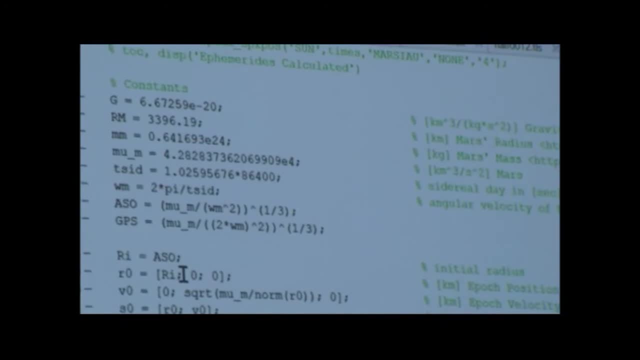 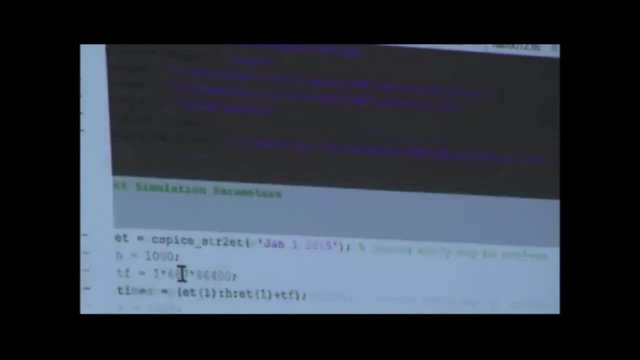 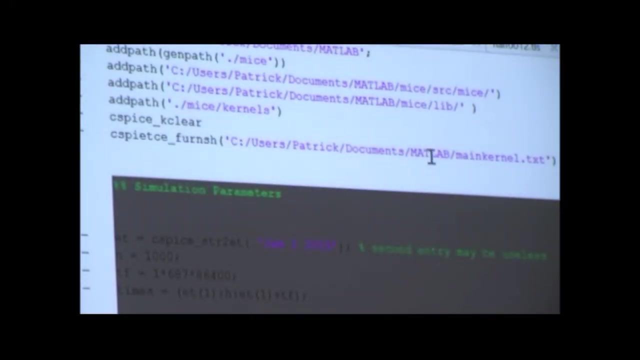 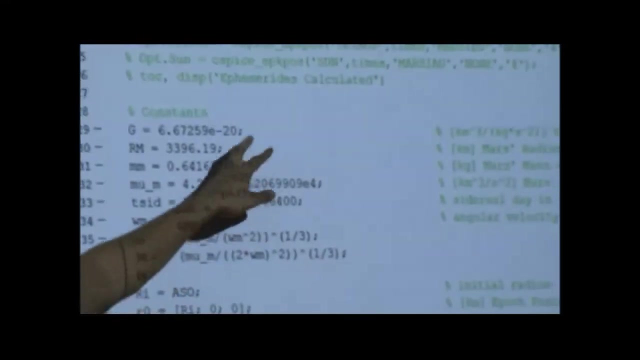 The frame I'm using is a Mars centered frame. It's an inertial frame at Mars called Mars IAU. I have it commented out, but I pull it. It's inside the function I'm using. Basically. I'm going to use this Cspice position kernel here. 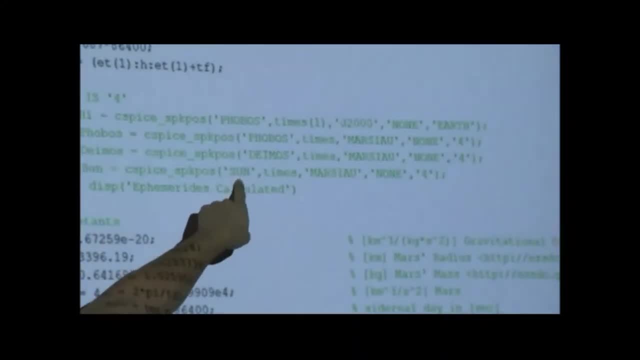 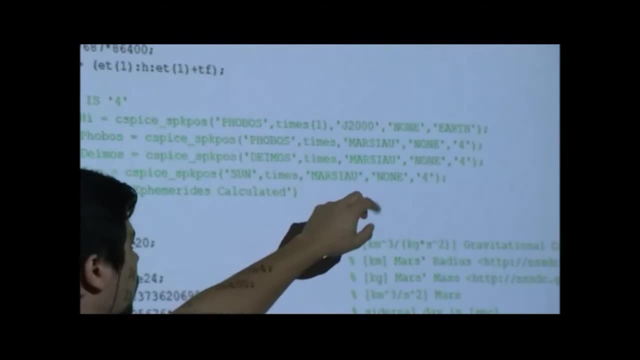 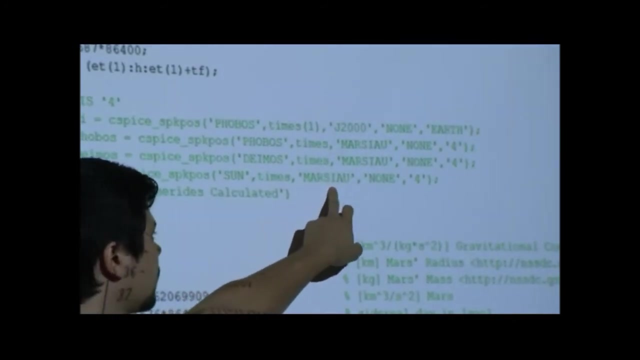 I want to find for this particular variable, the position of the sun at whatever many times, Like a time window here In reference to: Well, in this coordinate system called Mars, IAU, this is an aberration correction. I always just leave that blank for now. 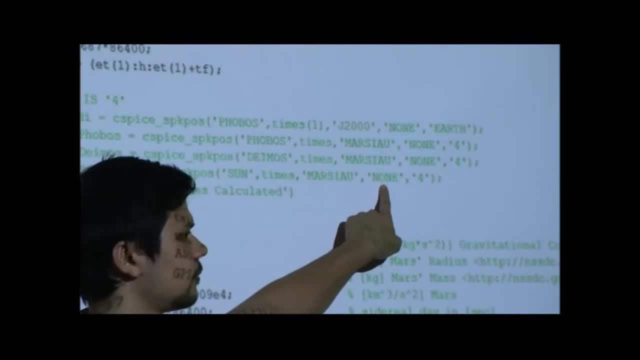 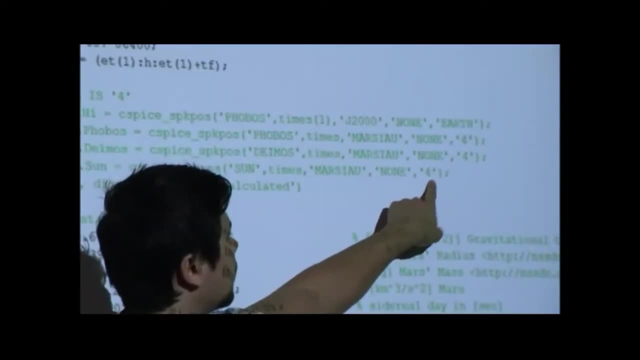 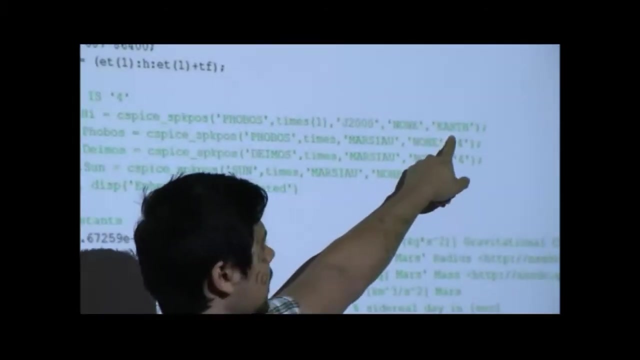 That's kind of a. It corrects for relativity and these times Like the time at Mars versus the time at Earth. This 4 is the number for Mars. You can see up here. I have Earth as my reference body. I could write: 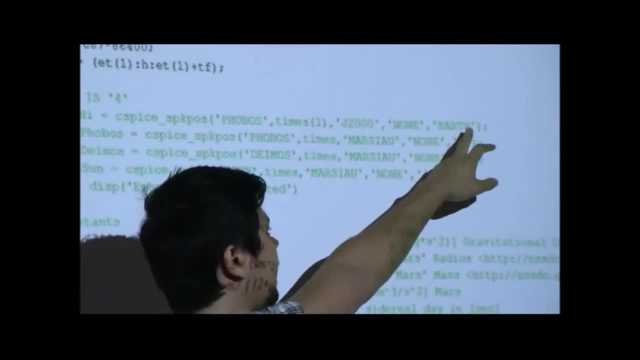 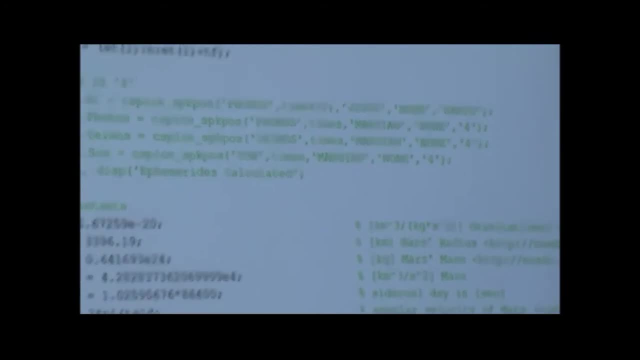 Its code is 399.. I could read the right Earth or 399 in here. Cspice will understand that I'm going to go ahead and put 4, because that's the identifier from Mars. What it's going to do is: 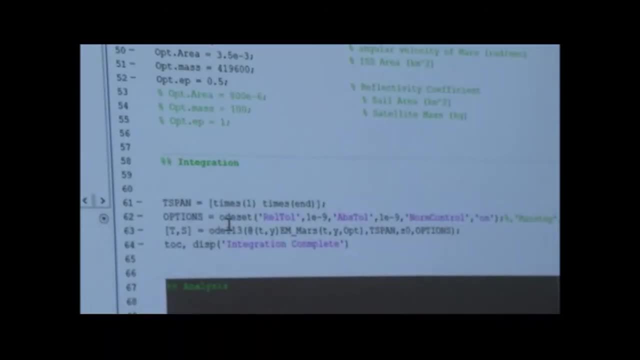 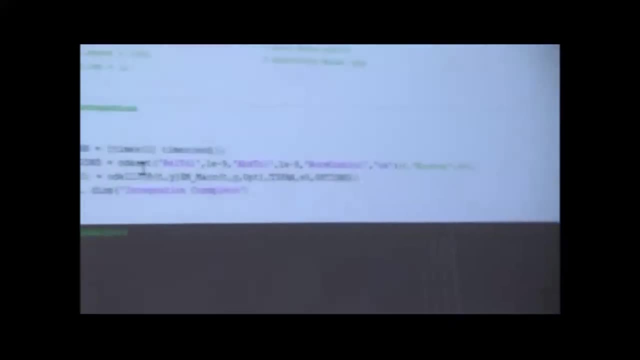 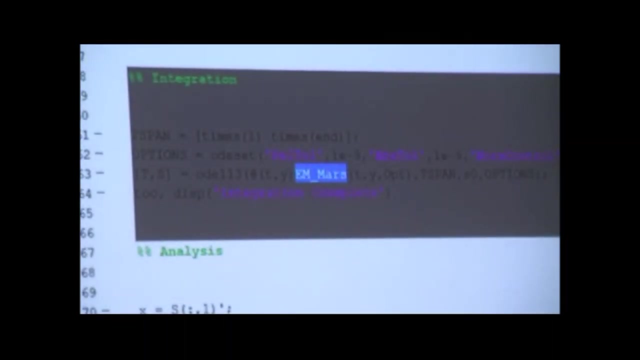 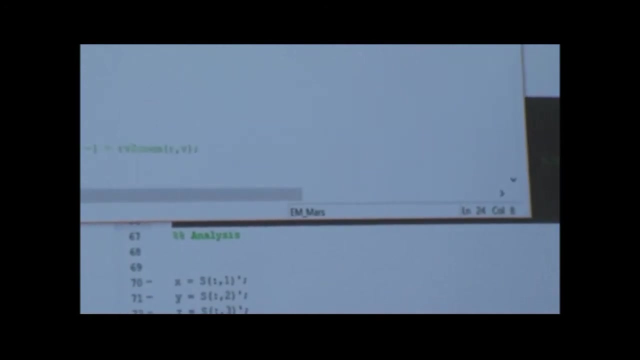 I'm using ODE113 instead of ODE45.. It's a different kind of integrator. It's got a predictor and a corrector, as opposed to ODE45, which just integrates. But I'm using this EM Mars file which I'll pull up here. 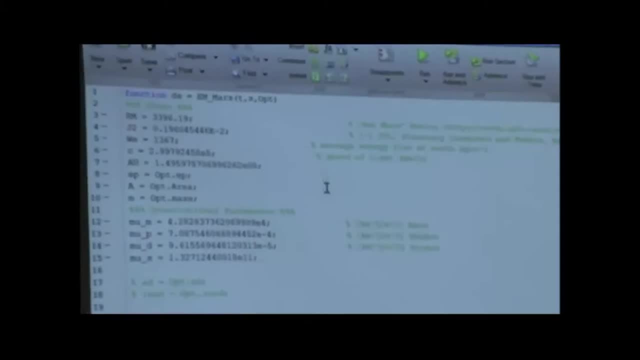 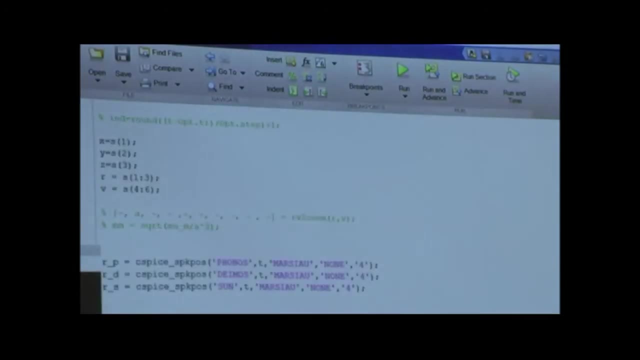 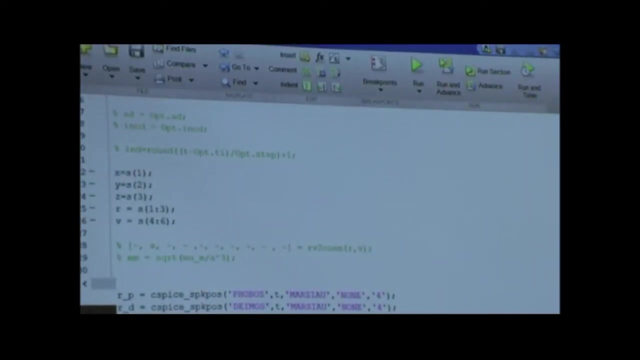 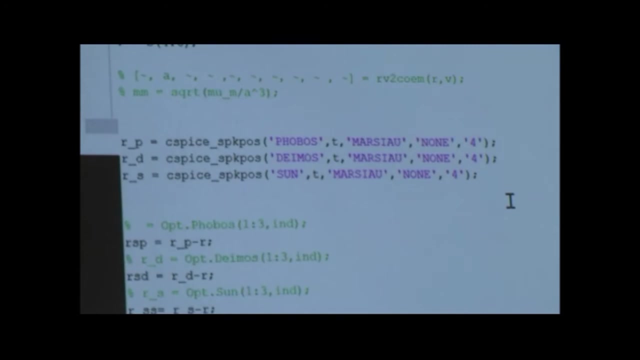 Cool, All right, It's not smooth. There you go Inside my equations of motion. I'm doing the long approach. I'm just going to, at every time step, get the accurate position of the Sun and the Moon at Mars. 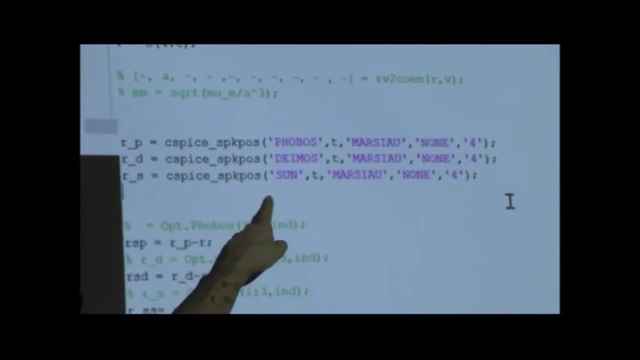 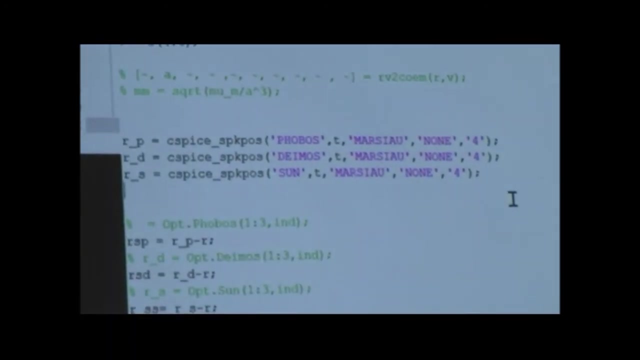 Here I'm actually calling Cspice, SPK position. I want the Sun information in this Mars reference frame at Mars for my integration time t. Then these are the forces I'm going to be having in my model. I've got a third-body acceleration from the Sun. 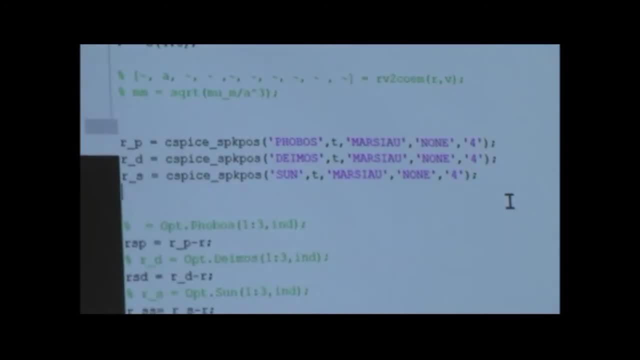 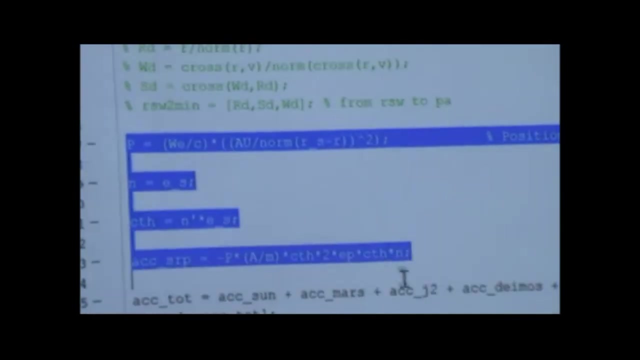 the two Moons, the standard two-body acceleration from Mars, and I have J2 in here as well. Just for fun, I threw in solar radiation pressure as well. That's what all this information is down here. We're just going to see what the orbit is going to look like. 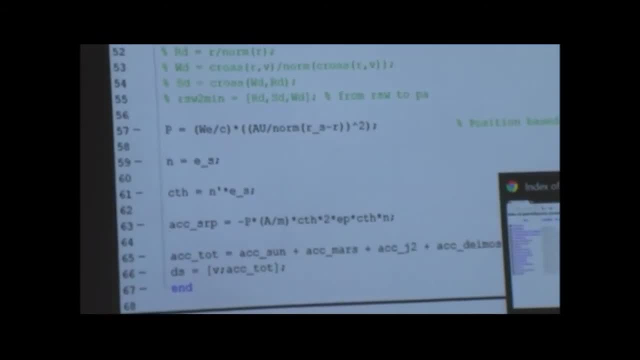 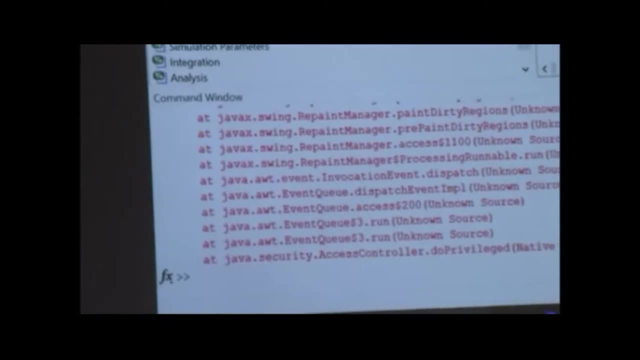 What the orbit of the ISS would look like around Mars at this 17,000-kilometer altitude. I decided, If I can, just second to second, if you want to say, that after we finish with the impulsive model, we're going to stop talking about all those additional observations. 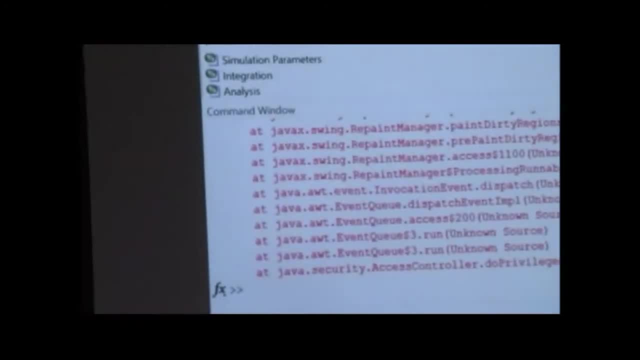 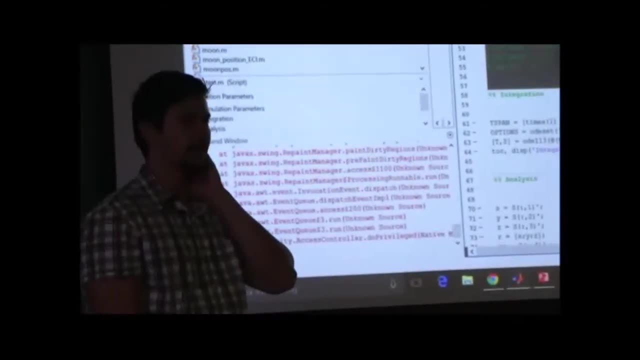 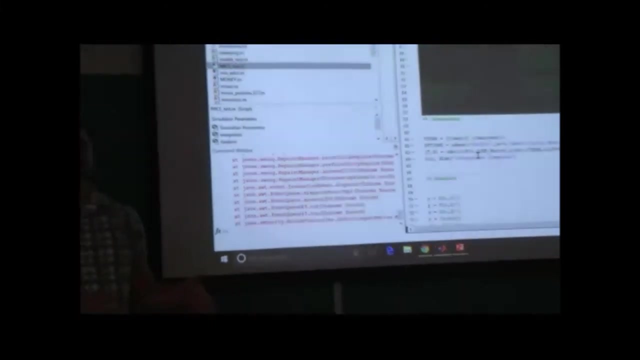 that you are thinking about? Okay, Did everybody hear that? Eventually, Right now we're just talking about two-body equation. when we talk about the force model, After we start talking about impulsive maneuvers, we're going to go into perturbations in better detail. 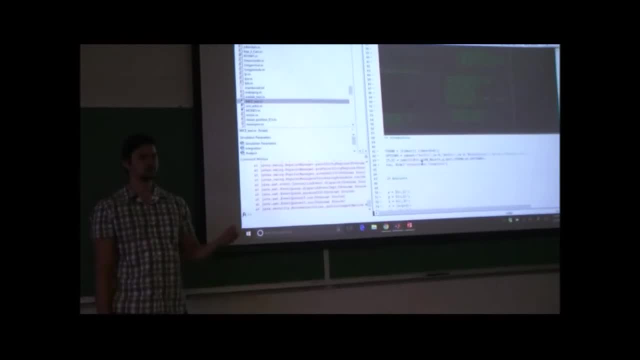 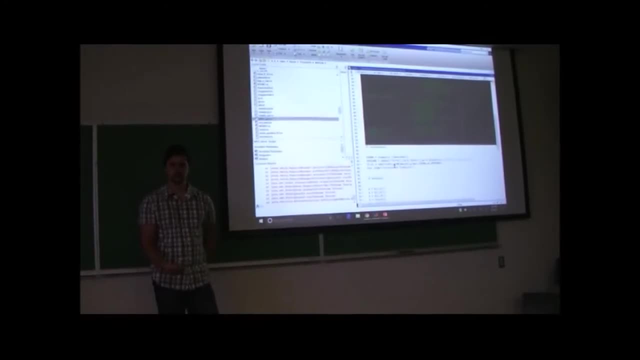 so you'll understand exactly how these extra perturbations affect the orbit. We'll go into more detail about J2 specifically, and we'll talk about these things called Gaussian variation equations, which kind of give you an idea of how the orbital elements will change. 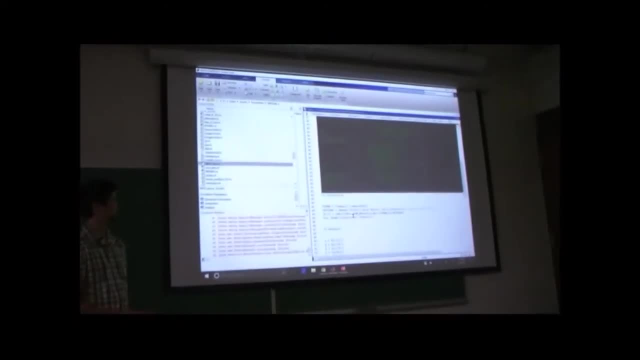 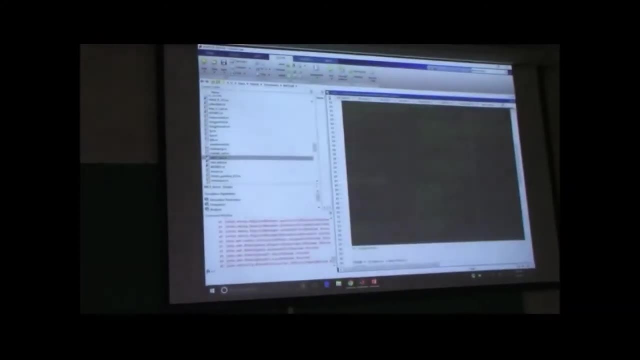 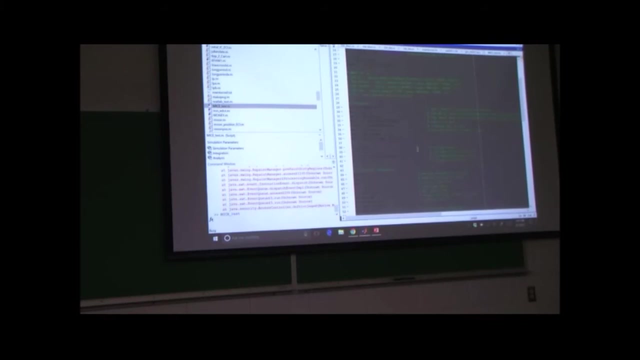 in time based on these perturbations, But right now, just trust me. Trust that this is working All right. Let's run this. This, I think, is just upset with the graphics card or something. Let's see While this is figuring it out. 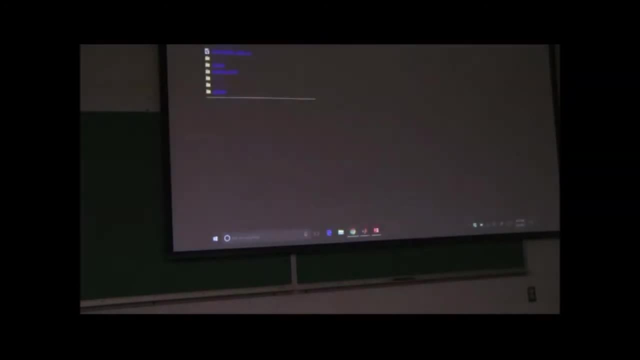 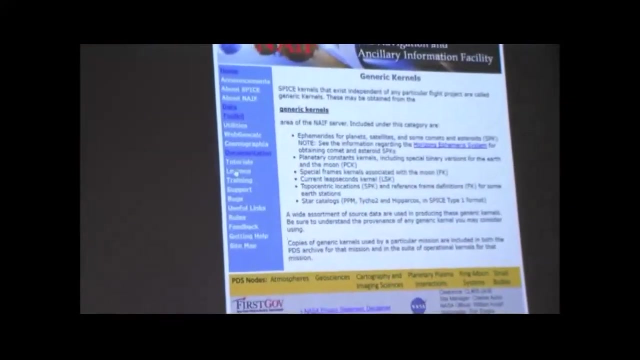 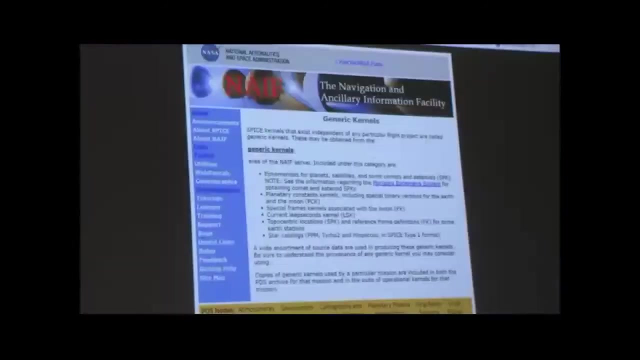 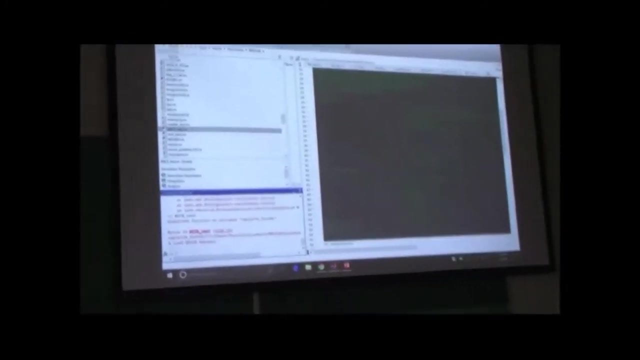 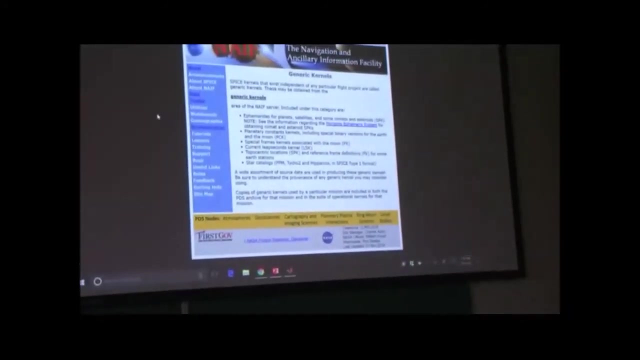 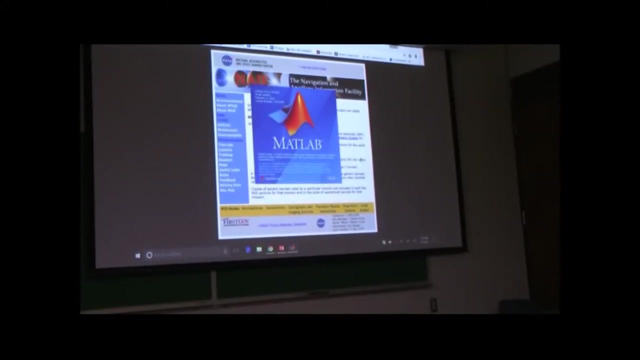 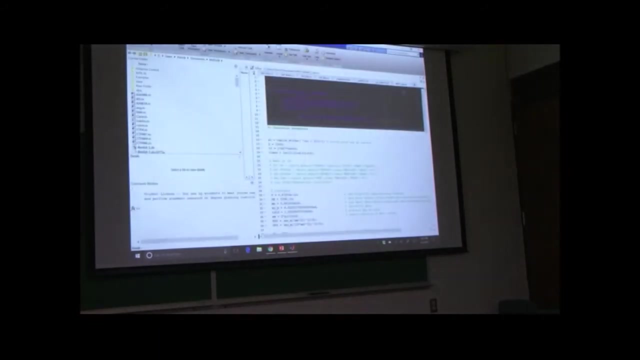 I'll go back to this website, Okay, So here's. Oh cool, That was fast, Oops. 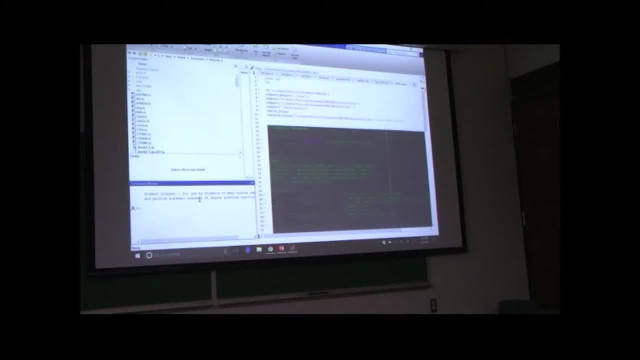 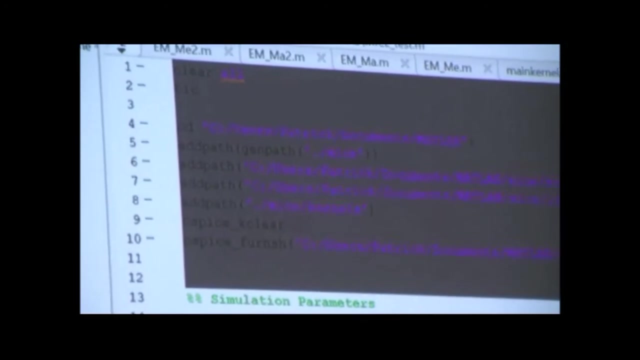 Oh yeah, I think I hit some keys when I was talking. Thanks, Harry, That was a good catch. That was a great catch. I wouldn't even have looked, Okay, So this should work now. 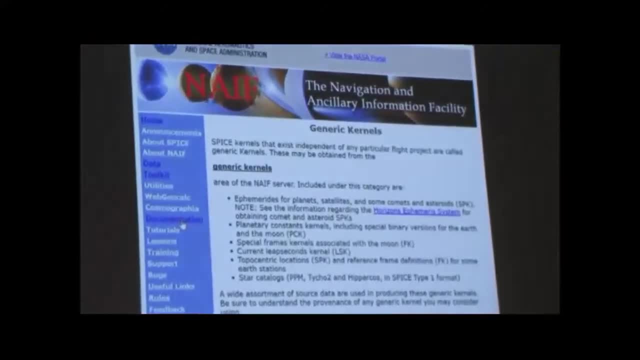 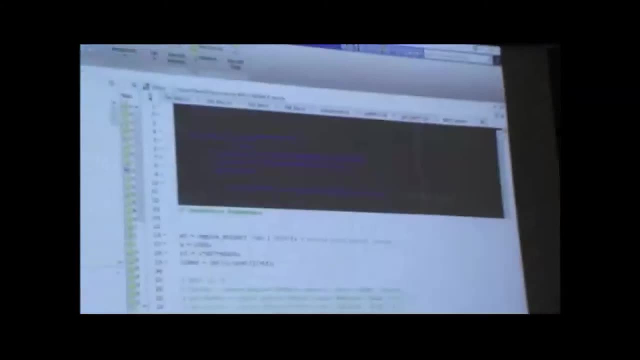 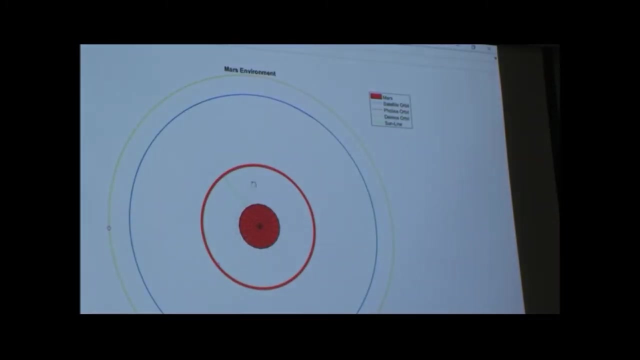 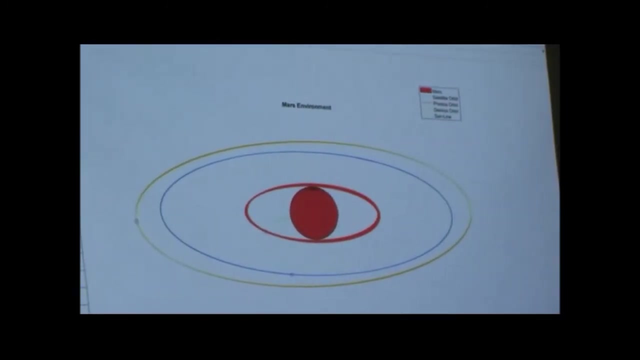 So back here, If you go to documentation, Sweet done, cool. So here's basically that plot that you saw in the PowerPoint. So this is kind of the result of the simulation I just ran. If you want to just look at the orbit, I have that here. 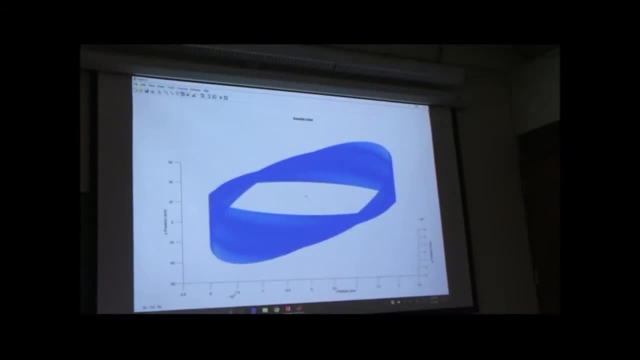 As you can see, we're not using any thrusters on board, so this thing is just floating around in space. but you can see, in the z-direction it's actually changing and that's due to the perturbations that we're talking about. 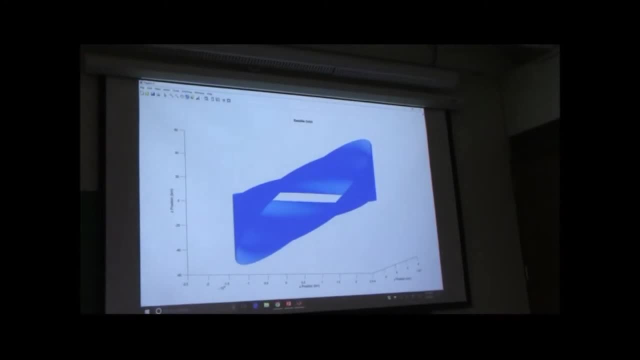 So in a perfect two-body model, this would just be a nice, pretty line, a nice ring. but because we added all that extra stuff in there, those extra forces, we get all these additional changes to the orbit. So I had this. 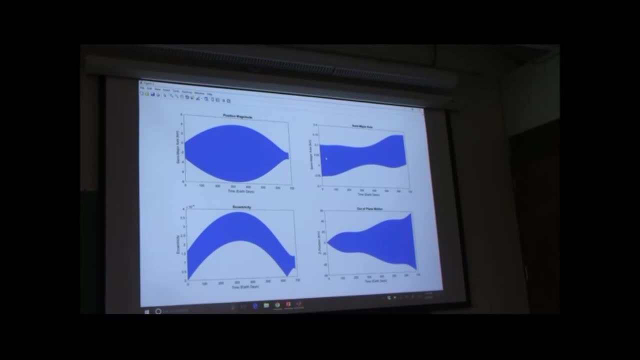 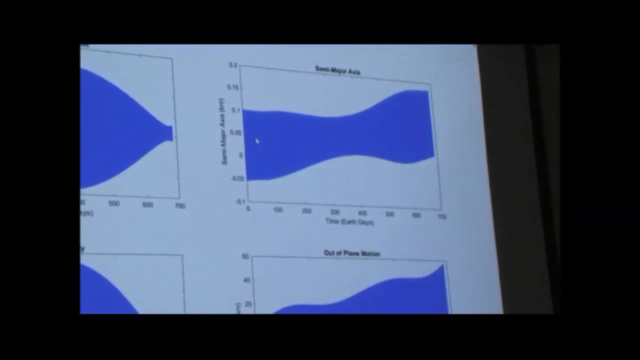 The semi-major axis centered at its original position. but you can see that because we have this change in the eccentricity here, we get a change in the semi-major axis, So it changes. it goes about 0.1 kilometers down to negative 0.05 kilometers from its. 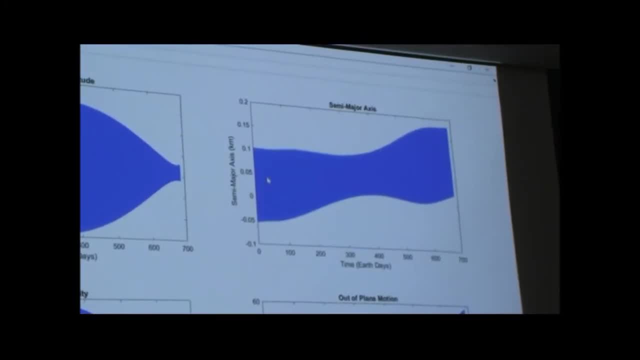 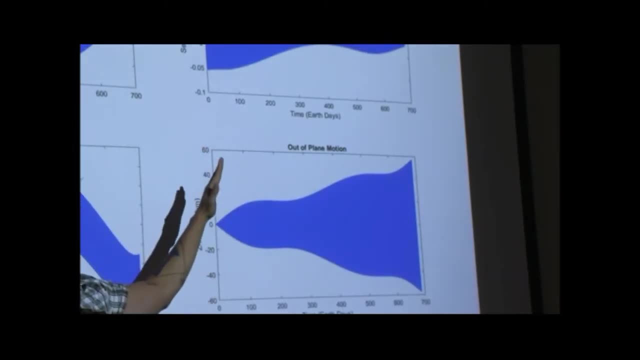 original position kind of oscillates around and we saw in the picture, in the orbit that I had displayed, you kind of saw that out-of-plane motion starting to rise. Yes, and that's displayed here as well. And that's all a result of these forces that I helped model with the SPICE tool kit. 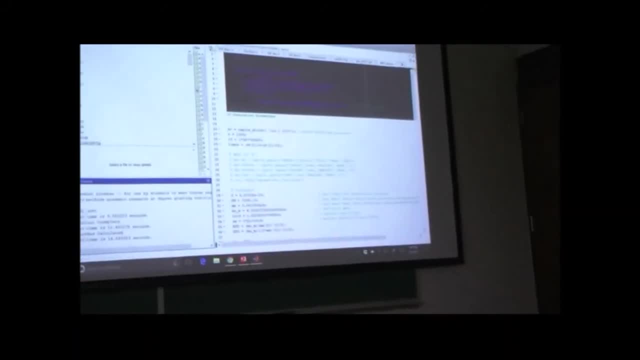 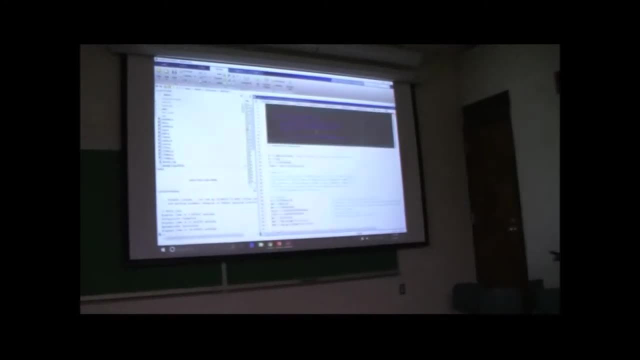 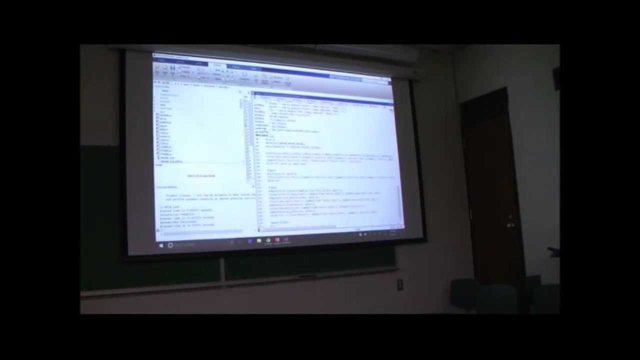 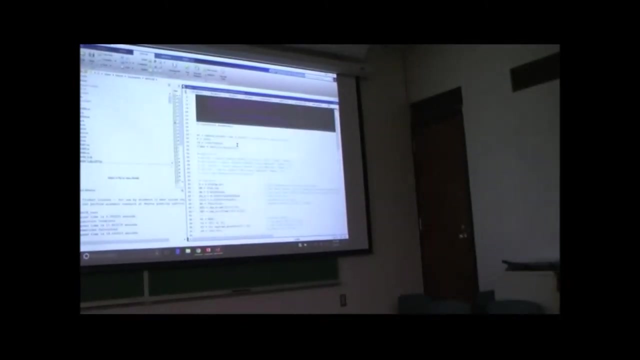 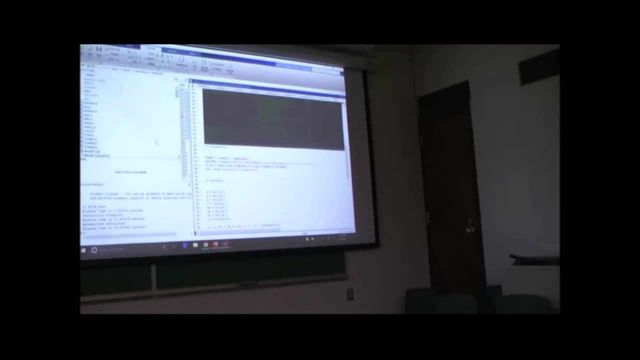 Okay, that works. Where is Now? if I decide I'm going to do this, I'm going to do this, Okay, If I decide to turn those forces off, you'll see a perfect ring. Yeah, Mars, all right. so I'm going to go ahead and turn those off right now. 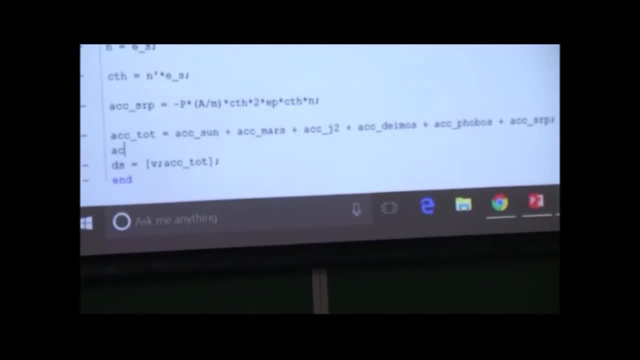 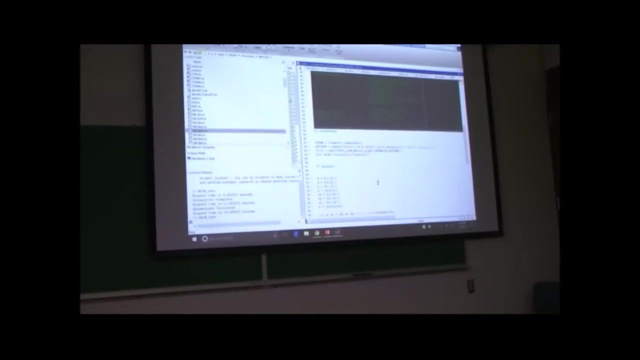 And we'll compare that to the previous plot. Okay, And we'll compare that to the previous plot. Okay, All right, All right. All right, So you can see it looks like there's a change here, but if you look at the order of magnitude, 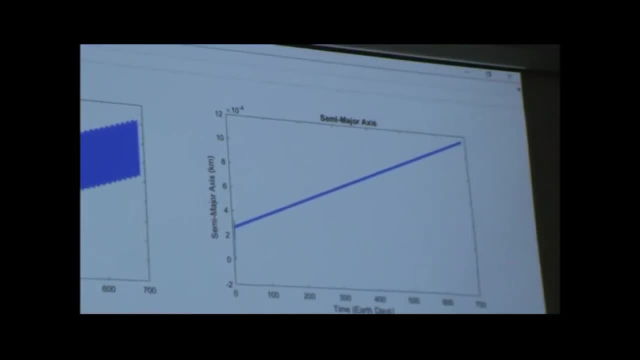 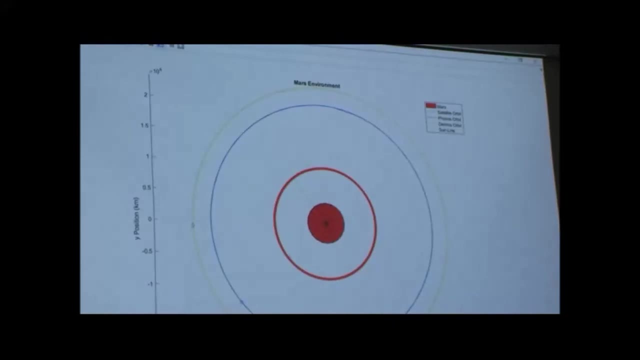 it's basically just machine error. Nothing's really happening. This should look about the same because of the scaling It does, but what we're interested in is this plot here. What do you know? So you can see the difference these perturbations have and you can see how we're able to use. 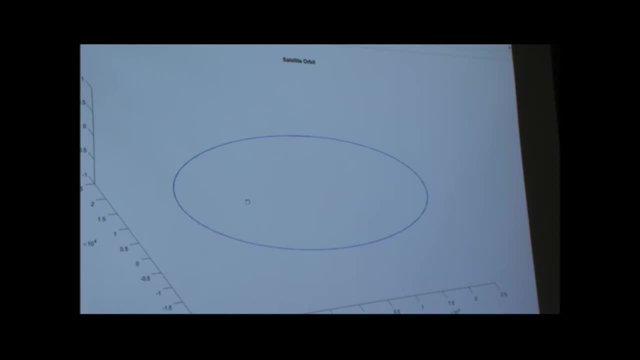 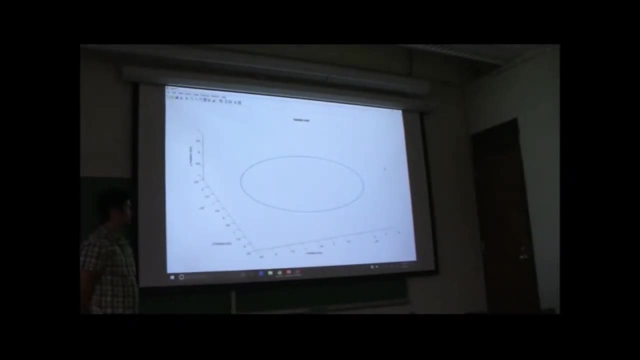 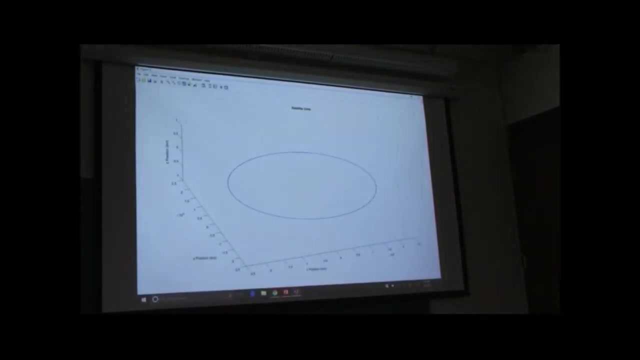 that with the SPICE Toolkit I would not be able to add these perturbations without the information about where the sun and moons are throughout the orbit to be able to get that more accurate plot that I have here. So you can see the utility of this toolkit here. 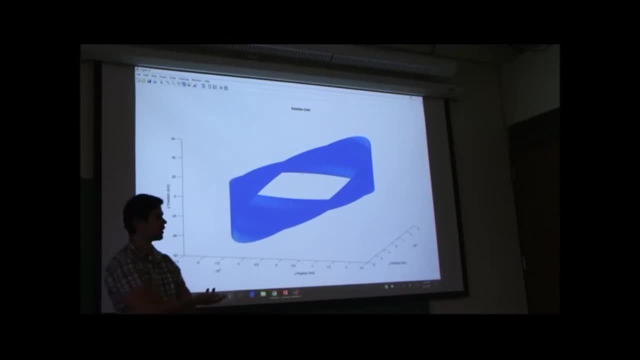 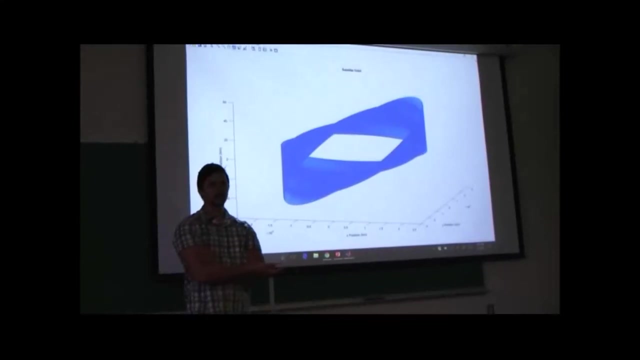 If you want to actually have a more proper mission design, to see how your satellite is going to evolve, you need tools like SCK, tools like MATLAB and an understanding of your dynamics model. But with C-SPICE you can actually put into practice these dynamics models. 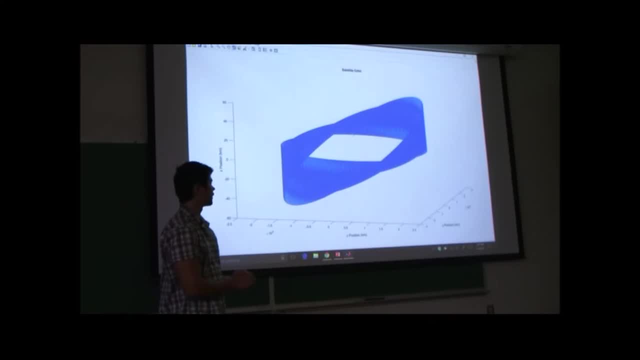 Okay, So you can get an idea of where these bodies are in reality, What some people do, just to get an idea of how these perturbations will affect the orbit. you can kind of fake a sun or fake a moon. Maybe you have an idea of how quickly the moon orbits around Mars. you can try to make 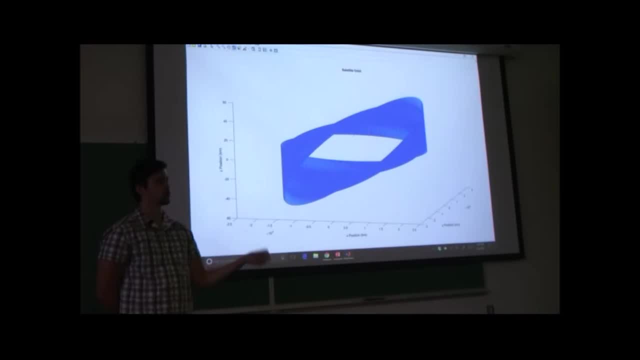 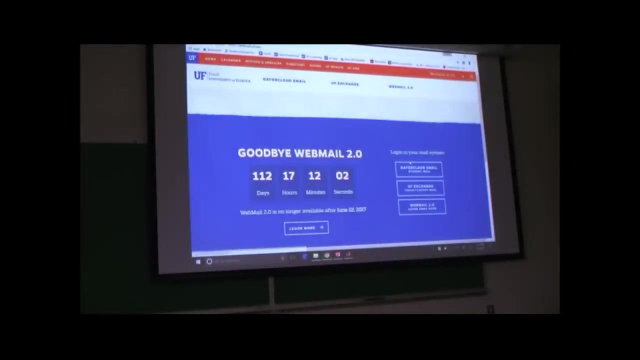 up a body, but it's not accurate to where the moon actually is, and that's why you use things like C-SPICE and STK. But yeah, I'll go ahead and pull that up right now And I put together an uncollected homework for you all to look at, if you want to try. 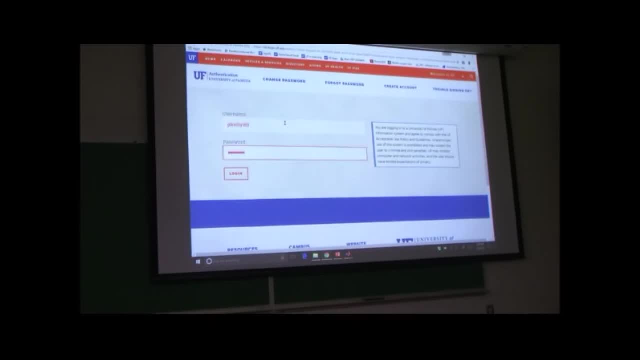 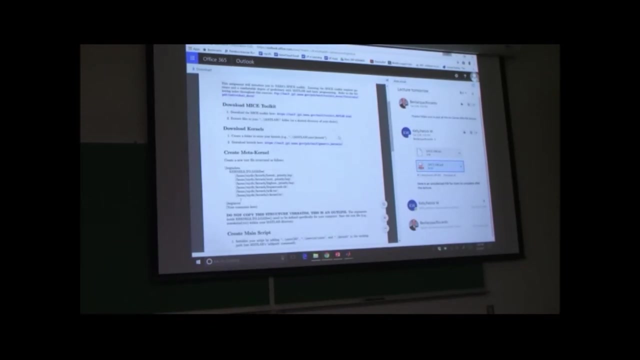 to play with this and I'll post it on Canvas here after class. Okay, Okay, Okay, Okay, Okay. So let's go ahead and download it. Oh goodness, I'm sorry guys. I look at scripts and I'm like what is this? 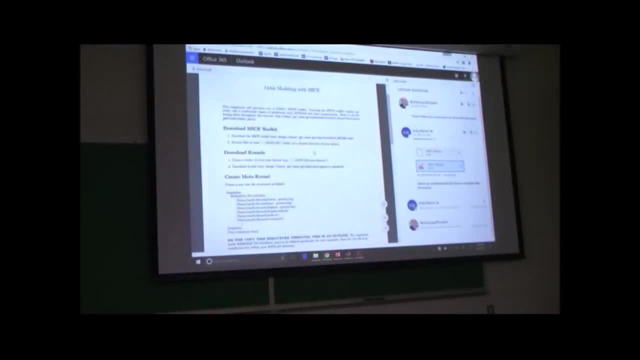 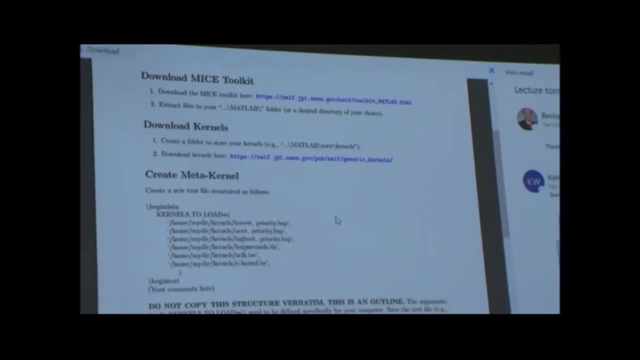 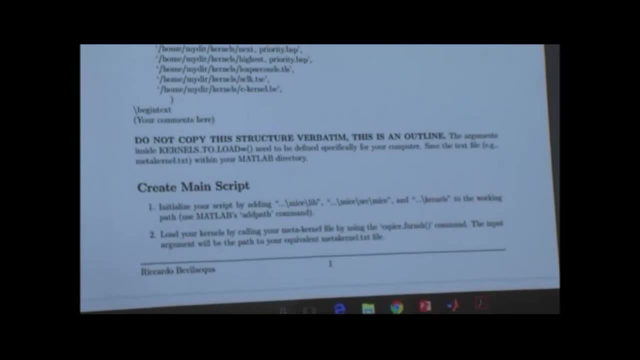 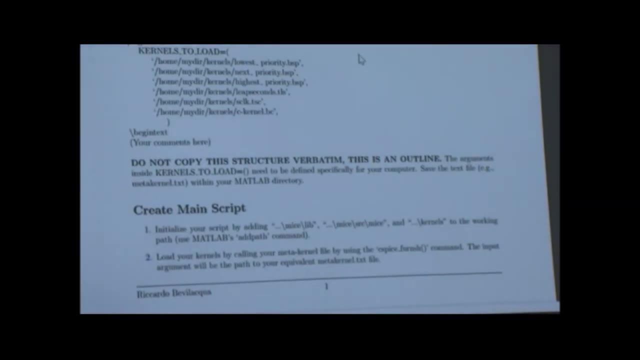 computer. I do a good job of demystifying the whole process so you can get this up and running in probably like 10 minutes. So here's instructions on how to load it up, But here's really the assignment down here. 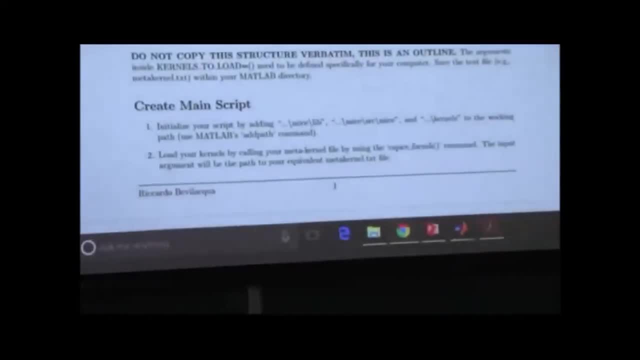 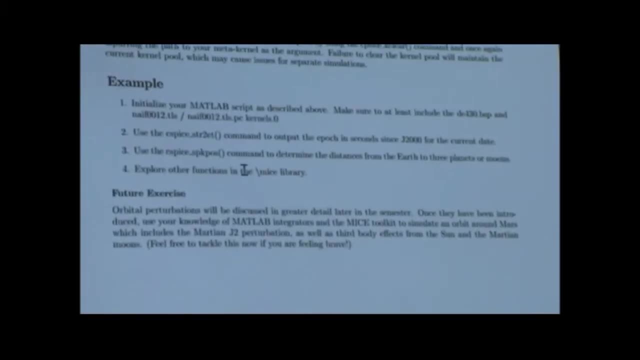 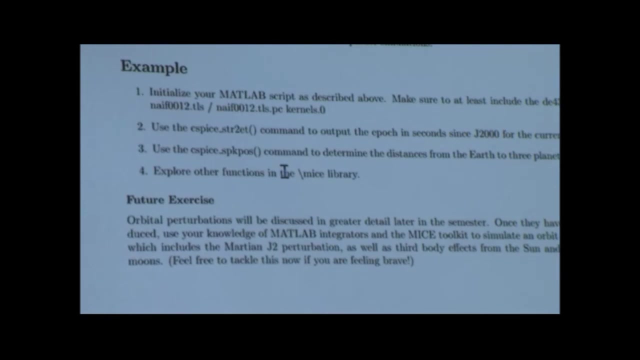 the assignment down here. You can use the orbit that you made for homework one and modify it a little bit to include- actually you don't have to use it at all. I kind of give you an instruction on how to use some of these functions to call sub functions in cspice. 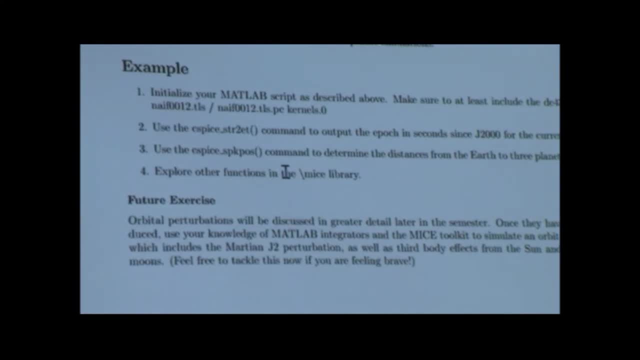 to get a position for where the moon is on your birthday, for instance. Maybe you want to know where one of Jupiter's moons is with respect to one of Mars moons. You can kind of play around with this function right here. You just put in a command and if you do help. 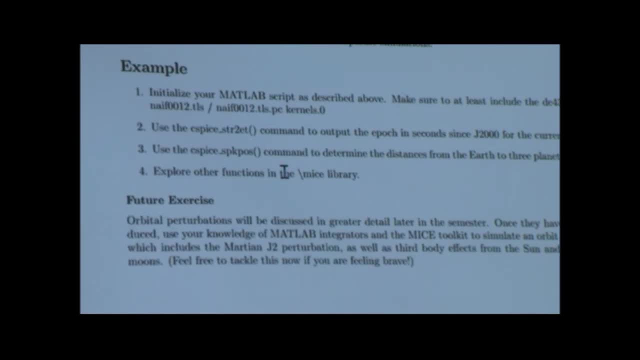 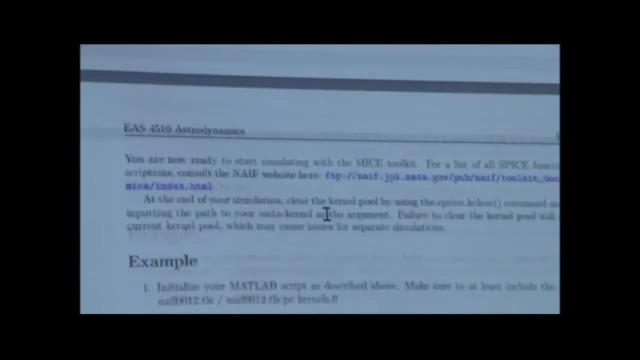 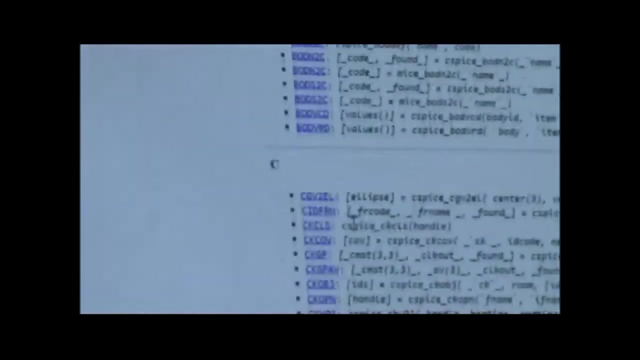 cspice sbk position. it will give you an instruction on how to place your inputs and I gave you some links. There are some links here that describe how to use these functions. If you go ahead and look at that uncollected homework, it will give you a nice guideline on how you guys. 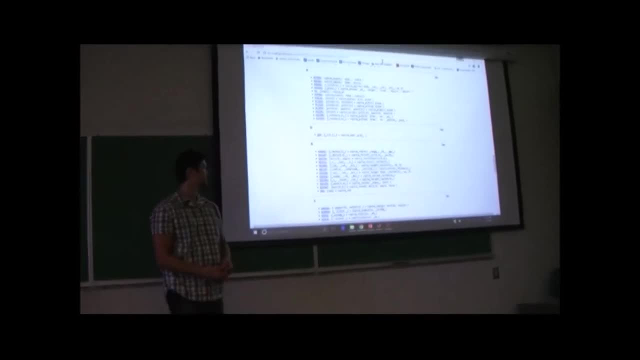 can start playing with this toolkit on your own. That's about it. Thanks a lot.